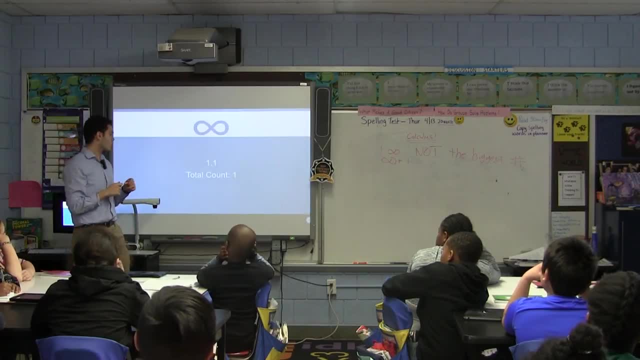 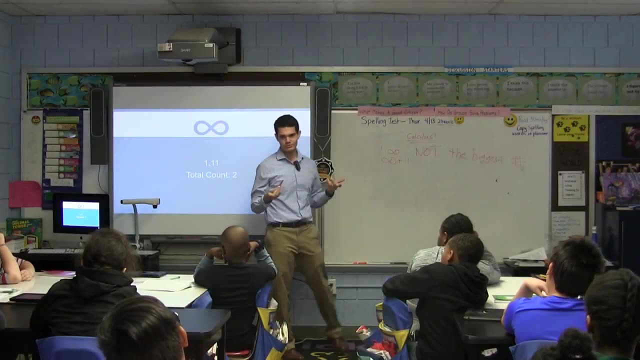 it definitely is between 1 and 2.. Do you all agree? Yes, So right now we have one number between 1 and 2.. 1.11 is also between 1 and 2, right? It's a little bit bigger than 1.1, right? So now we have two. 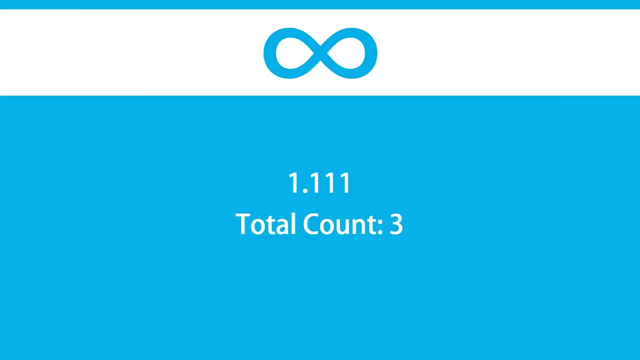 numbers that are definitely between 1 and 2.. 1.111.. This is also between 1 and 2.. So if we keep adding ones, that's what this dot dot dot dot means over there. that means: 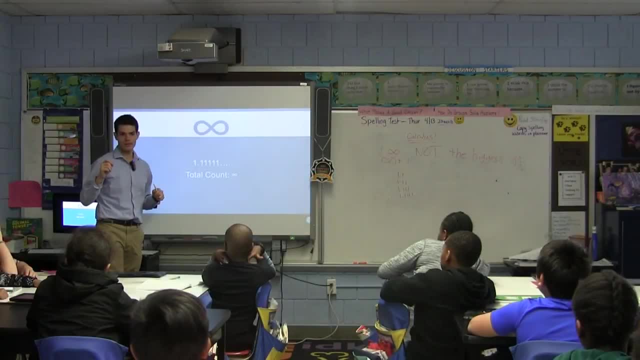 we can just keep adding one on until the end of this number, forever. And every single time we add one on, the number gets a little bit bigger, right? So it's a unique number. It's a different number- that's between 1 and 2- every single time we do this, And if we keep, 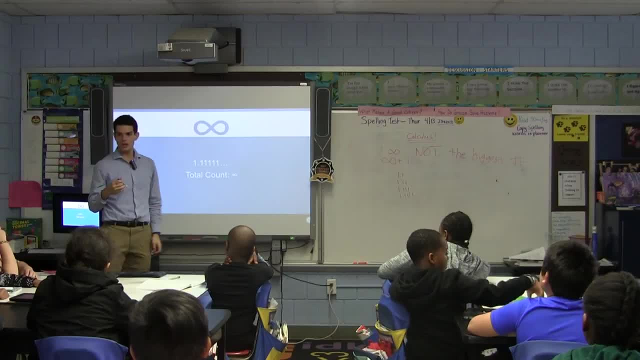 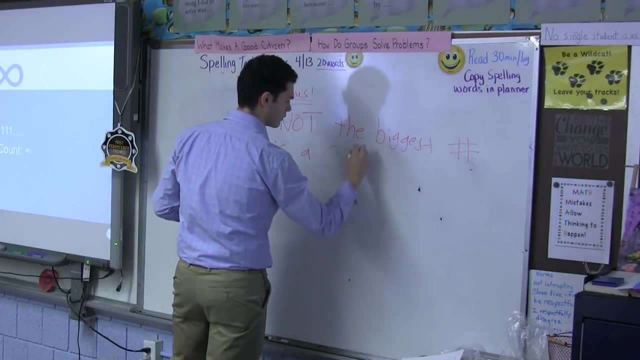 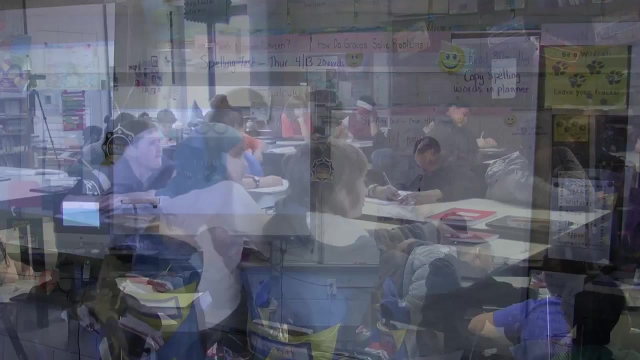 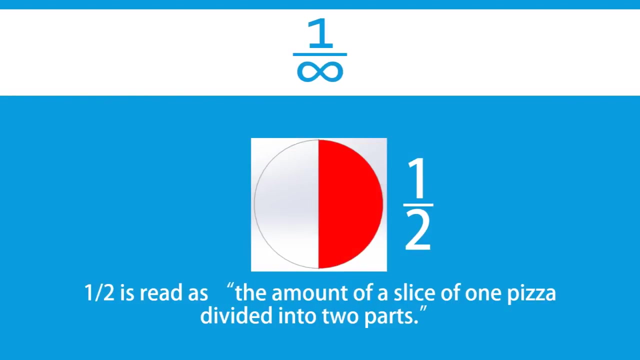 counting these numbers, as in how many numbers are between 1 and 2, we'll never end. That is infinity. Infinity is a concept, And this is crucial to understanding not just infinity, but also for calculus. Let's talk about 1 over infinity. If I have 1 over 2, we have this one pizza, we cut it. 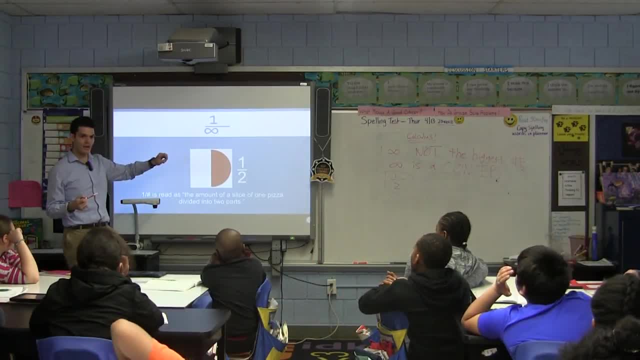 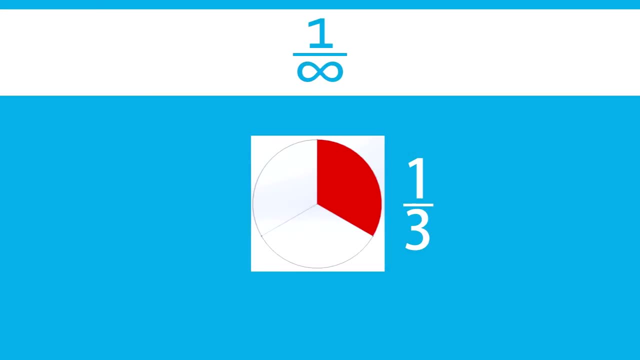 in half. and this red right here is the amount of my one slice. We all agree, Yes. So now let's go to 1 over 3.. We have this one pizza and we divide it into three equal slices. This red slice is the amount of one slice. And now, if we divide it into four, 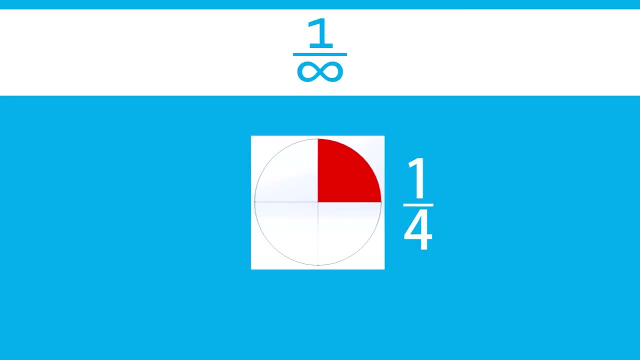 what do we notice? It gets smaller. It gets even smaller right? So when we have 1 over 5, it's a little bit smaller. 1 over 6.. 1 over 15.. Let's look at 1 over 80.. 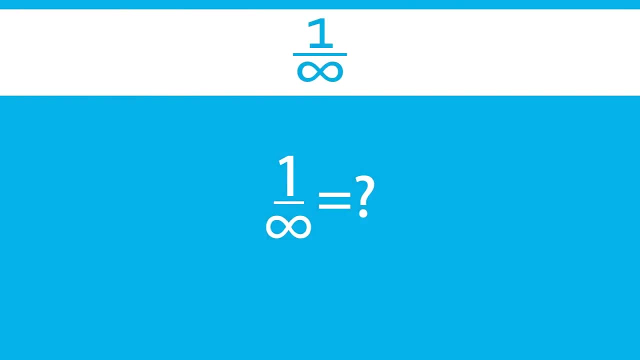 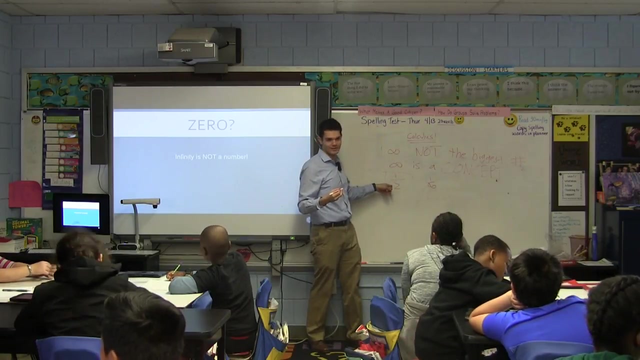 What would happen if we go to 1 over infinity? The question is, is it equal to 0?? So remember that infinity is not a number. So 1 over infinity doesn't represent anything. Remember, we had to have a number on the bottom of this thing. right, We have to divide it into a. 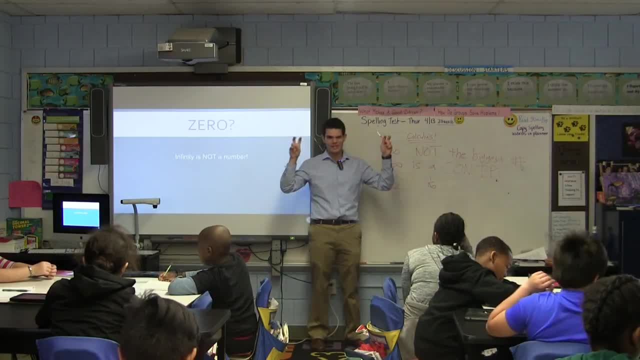 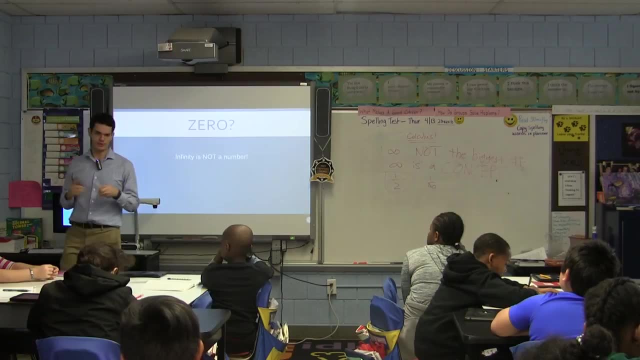 certain number of slices And if we divided it by infinity? to me that means nothing. But what does that mean about our pizza slice? Well, we said it's not equal to 0, but what we can say is that 1 over infinity. 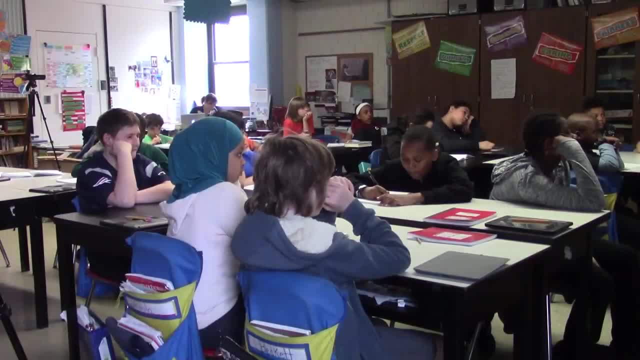 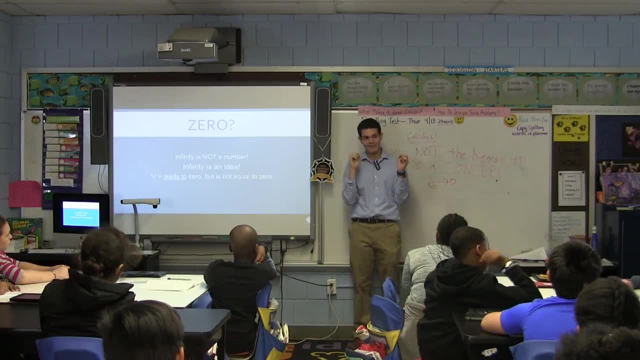 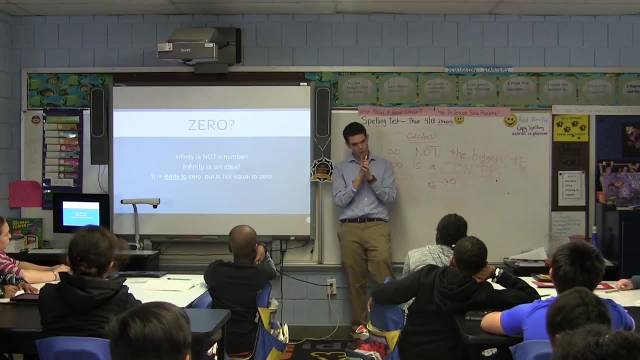 goes to 0. When we increase that number on the bottom, our slice gets smaller and smaller and smaller. And if we keep doing that forever and we keep adding 1 to that, bottom number is getting closer and closer and closer to being nothing. but it's never equal to nothing. 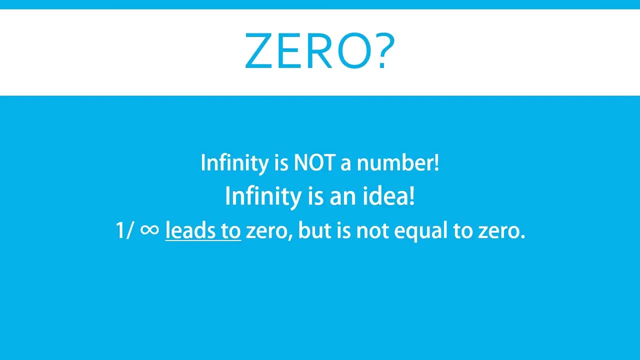 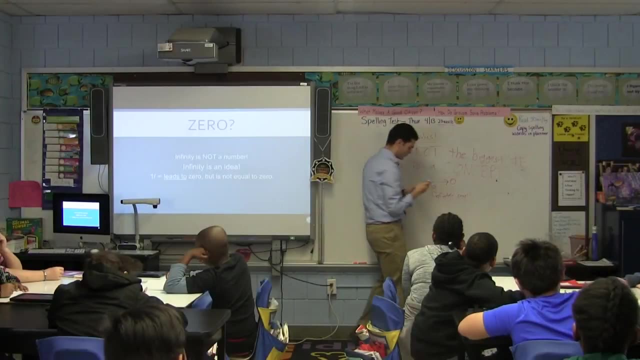 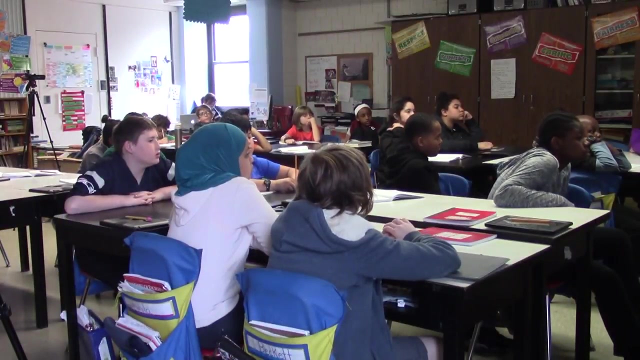 What this is called, and this is important. this is infinitely small. One. over infinity is an infinitely small number, just like infinity is an infinitely large number. Let's move on to something that I know you're familiar with, area I want to talk to you guys about. 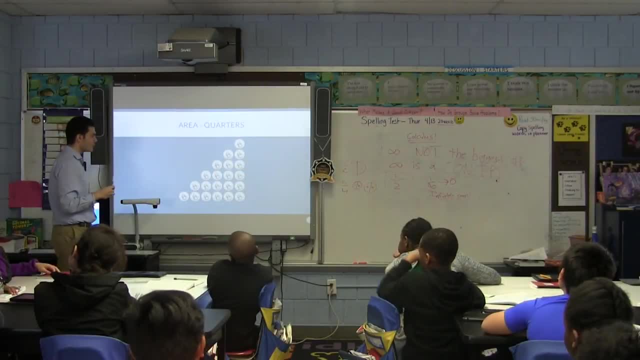 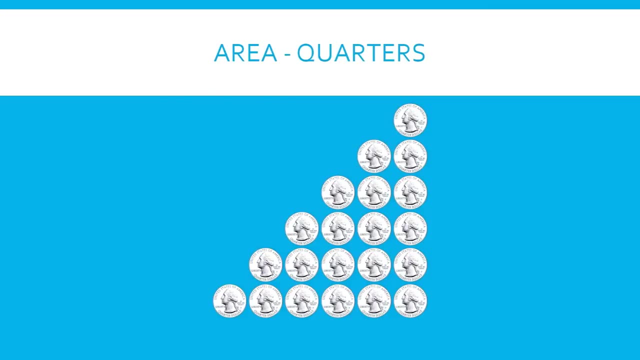 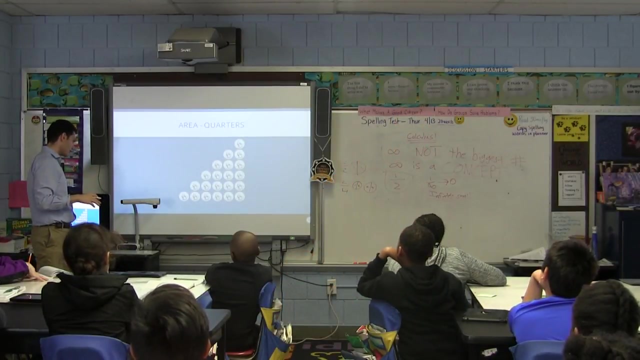 an interesting way to take area. Let's say we're trying to calculate the area of a triangle. A way that we might be able to do it is by taking something whose area that we do know and filling our triangle with it. Let's say we have our quarters stacked up like this: 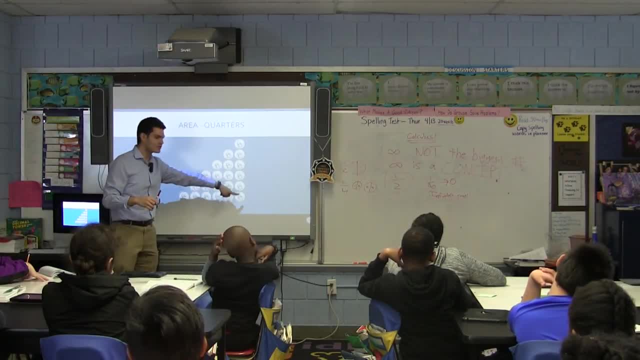 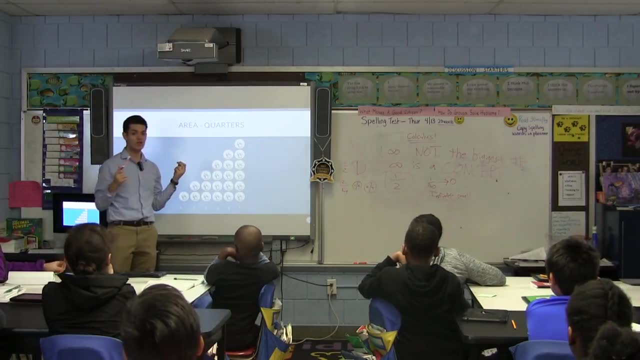 We want to say what is the area of a triangle that has this shape? Well, let's count the quarters and say how many quarters fit into this triangle. One way we can do this: we can count it just by going one, two, three, four, five. We can. 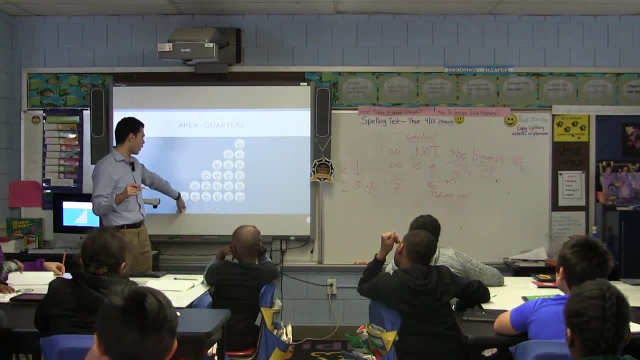 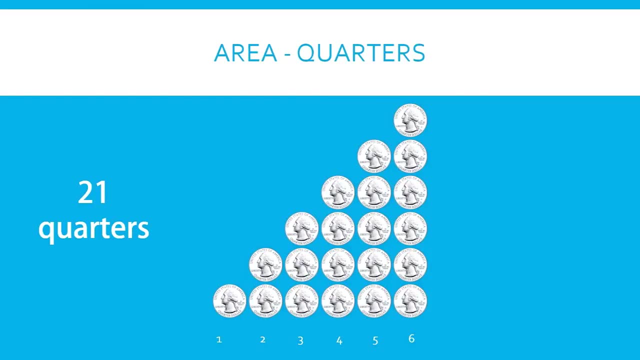 do that, but the way I want to talk about doing it is to count all the columns. If we count all the quarters, we add one plus two plus three, we get 21. quarters are shown right here. We can say that our quarters roughly fill this shape and that there's about 21. 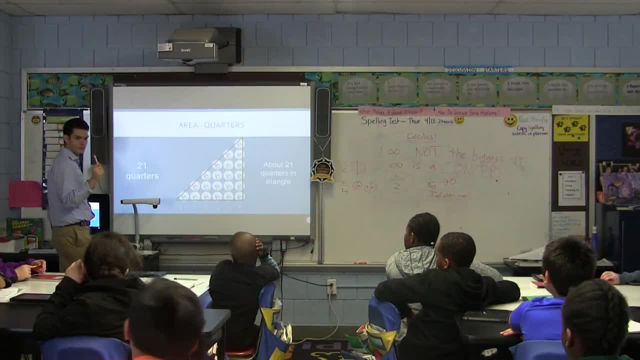 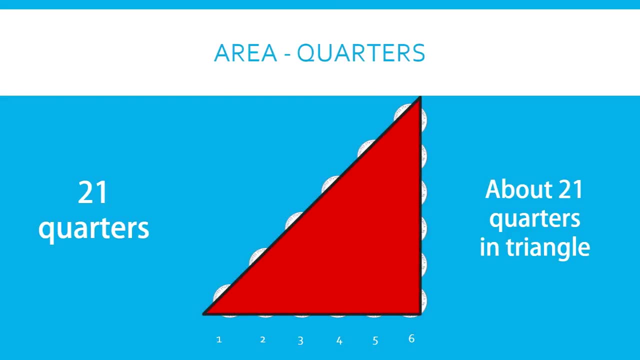 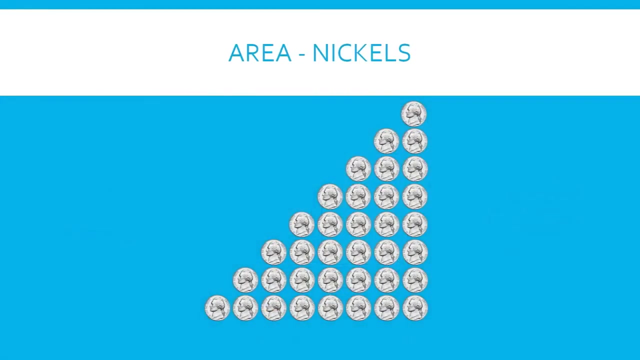 quarters in this triangle. If we fill this triangle, the first thing I wanted to show you guys is that there's a little space in here Where the quarters don't quite touch. If we fill the triangle in, we see that there's a lot of overhang on the quarters. How can we make this a more accurate measurement? 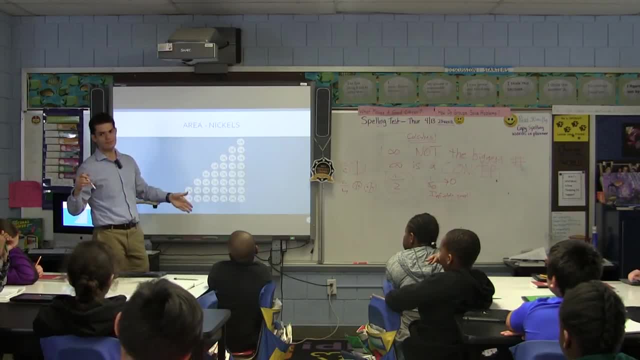 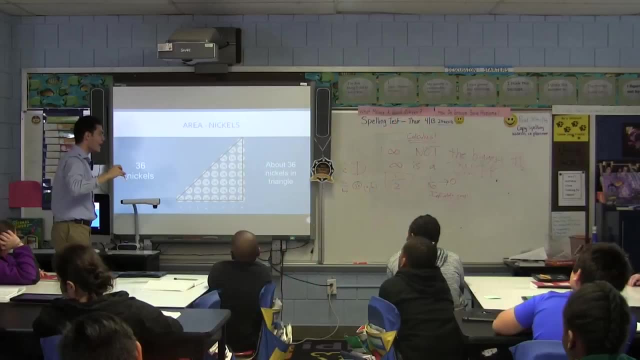 Let's use nickels now. Now we have a lot more columns. What we can do is we can add up these columns again and say, okay, well, there's 36 nickels here. Now, if I asked you how big is this triangle? what would you say? 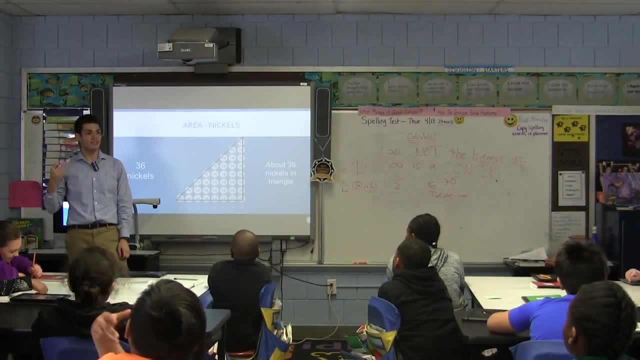 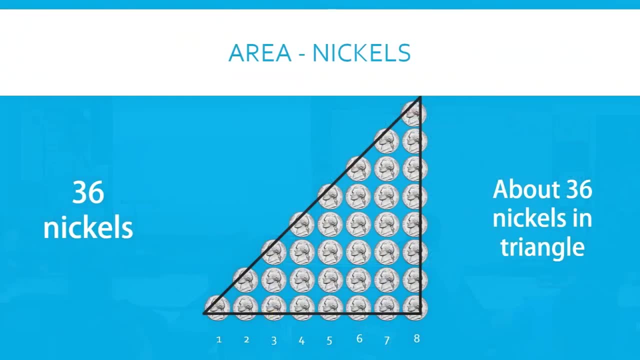 About 36 nickels. Again, we did this by counting up all the columns. Now, if we look at the inside of the triangle, the space in between the quarters are a little bit less. There's not as big of a gap between the coins, making it slightly more accurate. 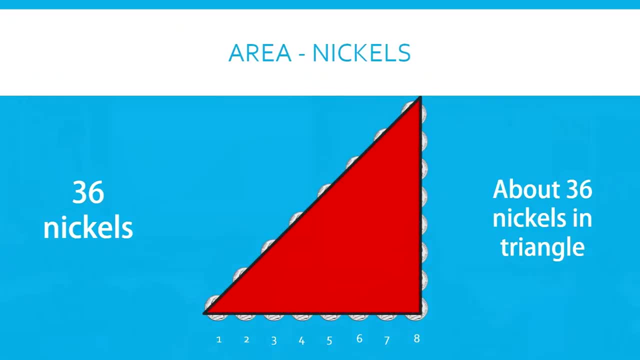 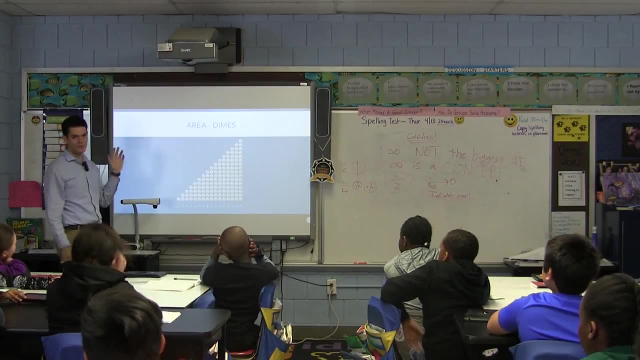 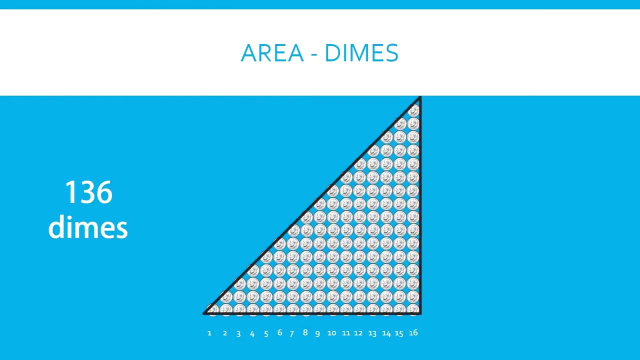 If we draw it, we see that there's a little less overhang. Let's go even smaller. Let's use a dime. If we count up all of the columns the same way that we did before- and there's a lot more columns, so it's a little bit harder- we get 136 dimes If we put this triangle. 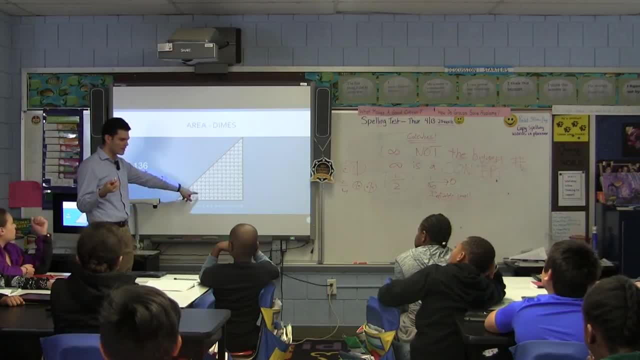 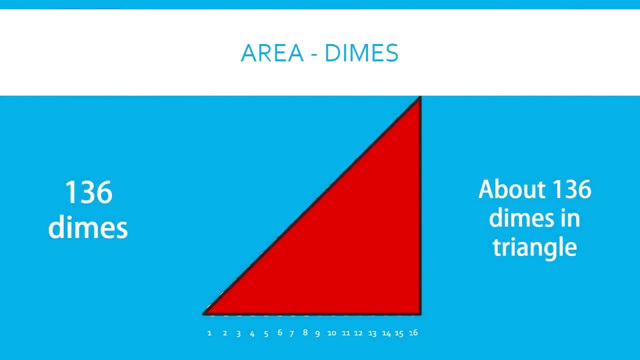 over. we notice two things. One, the space is really small now compared to the quarters. It's still definitely there, but it's definitely smaller space. If we fill this triangle up, it almost looks perfect. We know that there's a little bit of space inside that we have to deal with, but as far 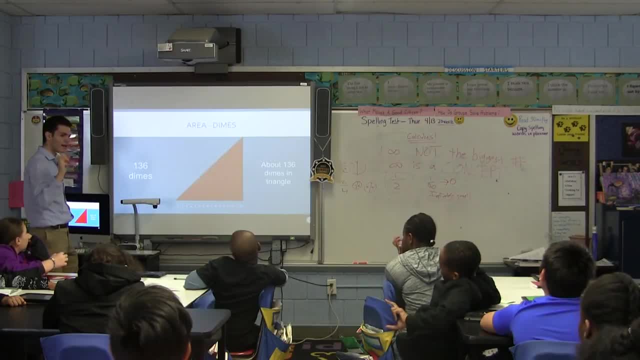 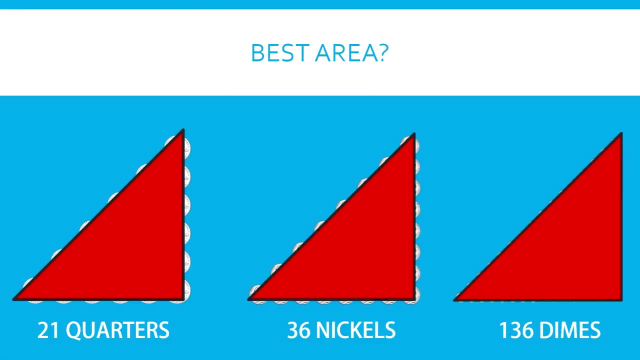 as overhang is concerned, it's pretty much gone. It's still there, but there's a lot less. Now let's compare the three triangles we just talked about. The dimes is definitely the most accurate out of these three, We all agree. 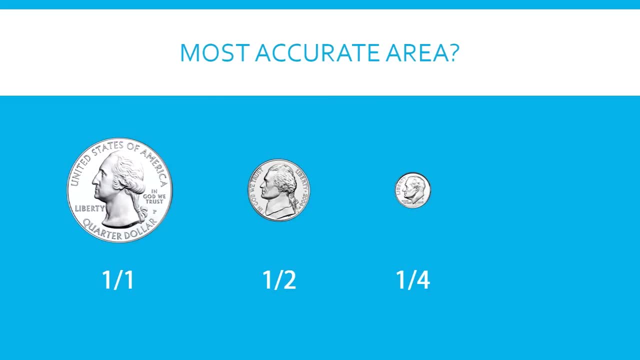 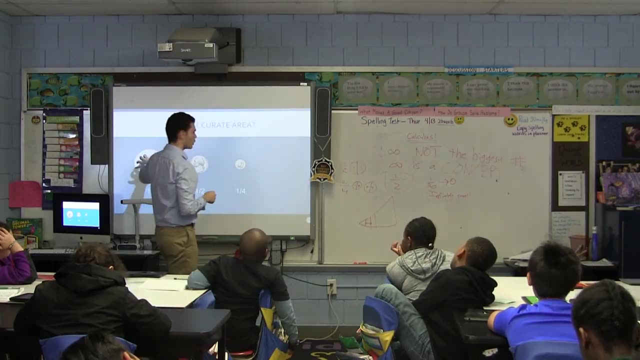 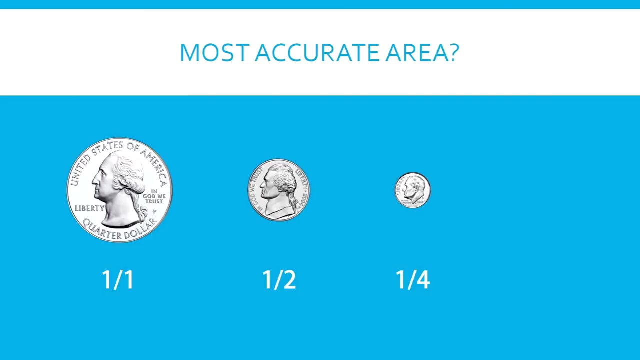 Yes, Yes. So we look at the columns that we used. The width of these columns is only as small as the width of this quarter or the coin. And so if we say this nickel has half the width of this quarter and that this dime has a quarter one-fourth of the width of this coin, we're 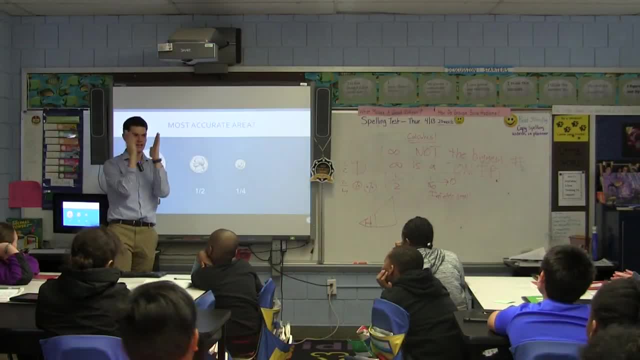 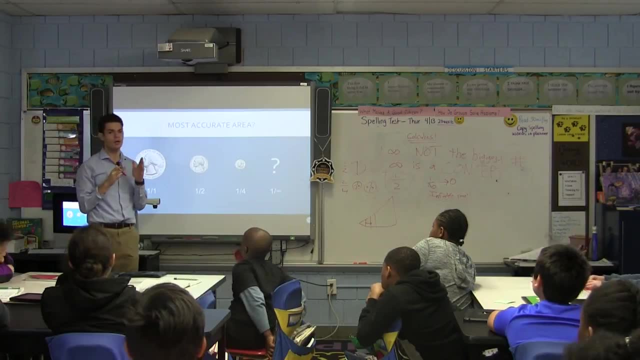 taking our column and we're making it smaller and smaller and smaller If we keep going on forever and ever and ever and making our coin smaller and smaller- which is not enough- and smaller and smaller, making the width of this column smaller and smaller by using: 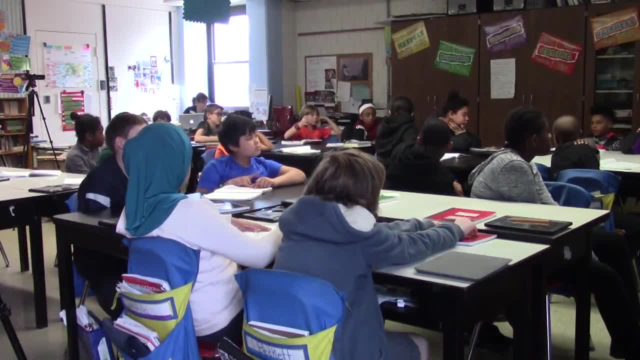 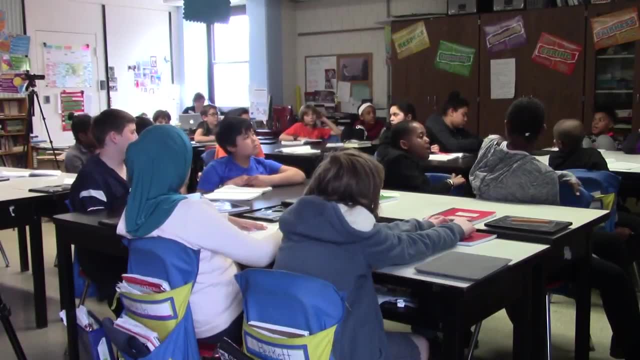 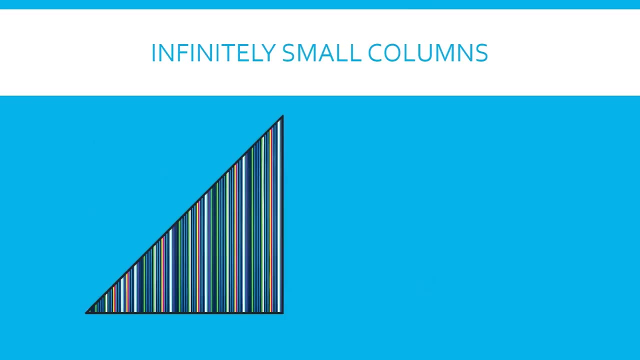 smaller coins. the accuracy is going to keep getting better and better, And if we make it infinity, our accuracy should be 100% eventually. So what would that look like? Well, let's take a look. This is a decent picture of what that might look like Now, obviously 1 over. 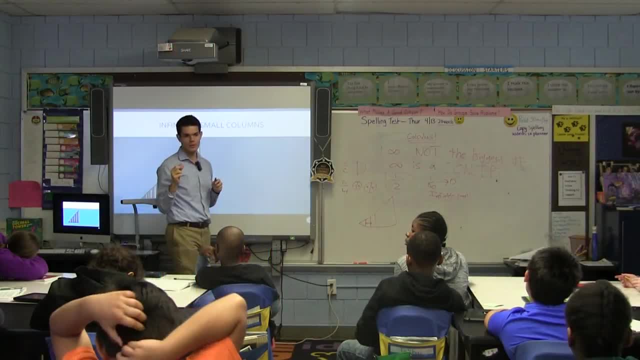 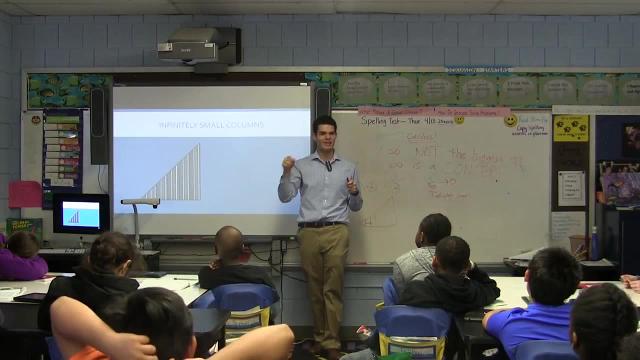 infinity is so small that we can't really represent it right. We can't make an infinitely small column on a computer, or even draw it, because we can always make it smaller. right, We can always add on to that infinity. But it might look something like this: And if 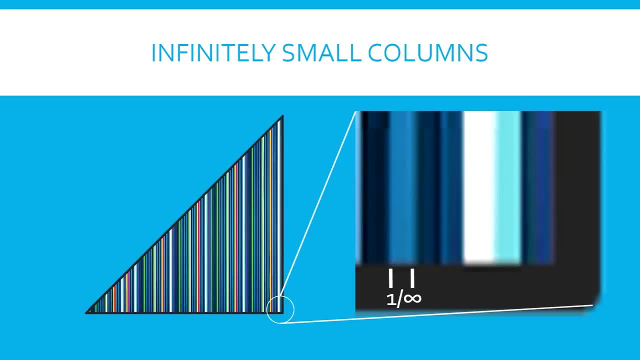 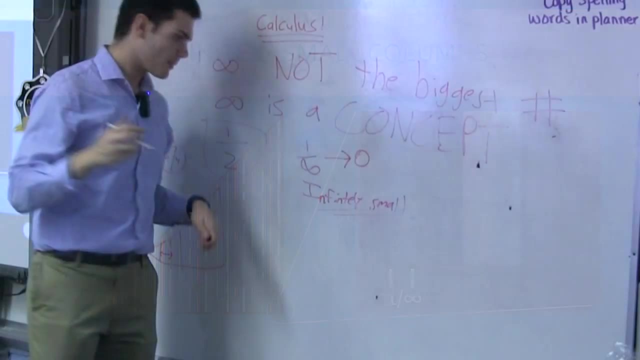 we zoom in to this corner over here we have these columns that go up right And imagine that these are the width of our infinitely small coins. If we add up all these columns, we would get the area of our triangle and it would be 100% accurate. This is one of 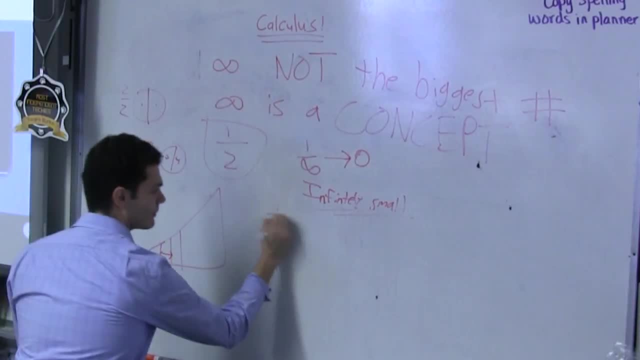 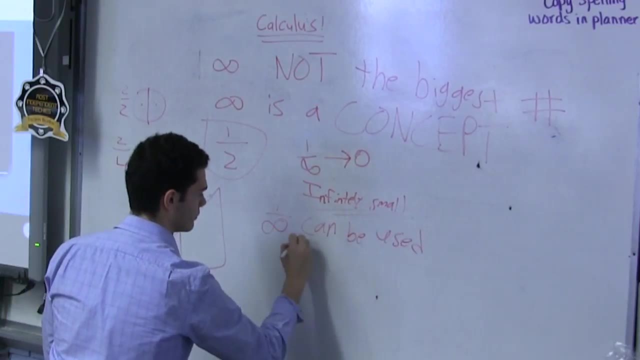 the big concepts that I want to address. One of the big concepts that I want to address is that 1 over infinity can be used to calculate area, to find the area, And this, this is huge, because this is one of the principles. 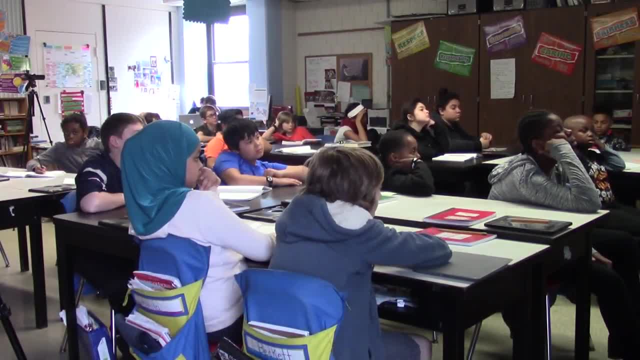 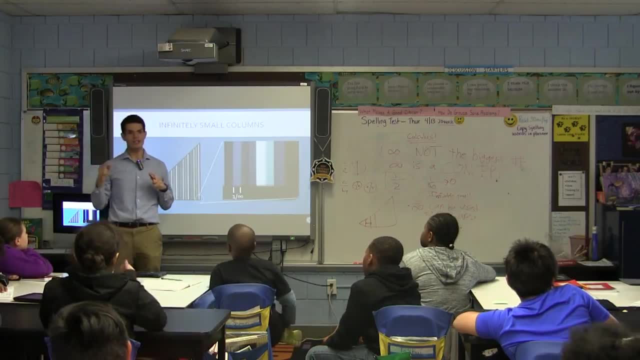 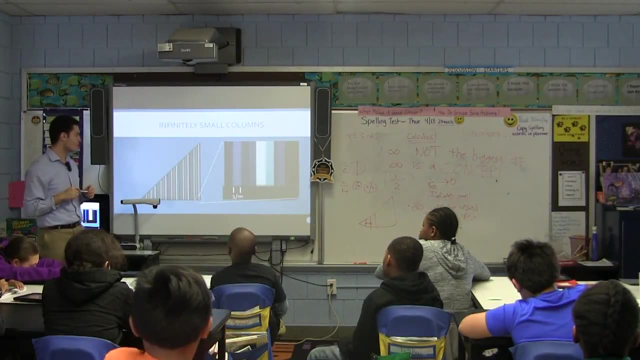 of calculus. This is the second- most- arguably first most- important idea of calculus is that if we use infinitely small columns, we can find the area of anything. Okay, I want to talk about another concept that's really important to calculus and that 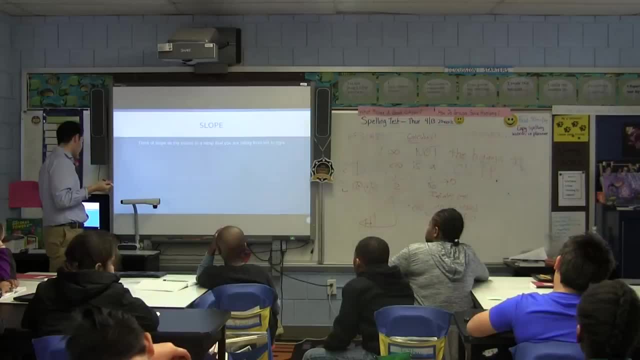 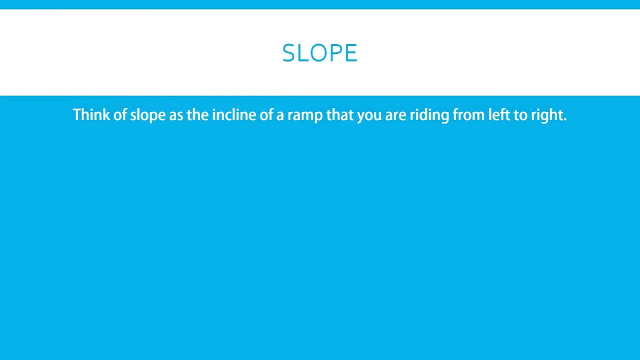 has to do with slope. Let's start by defining what slope is. So when I think about slope, what I think of is the incline of a ramp that you're riding from left to right. So, for example, if we have this guy over here, he's on a skateboard, he's going up this incline, he's going left. 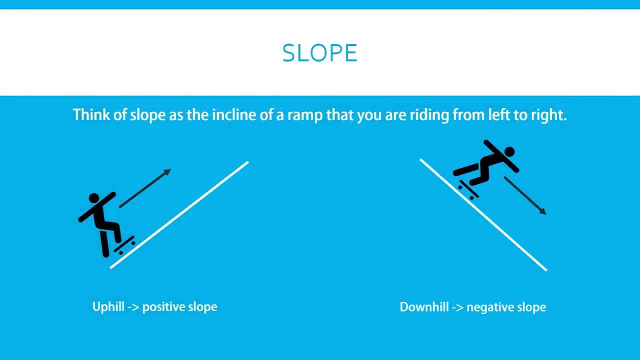 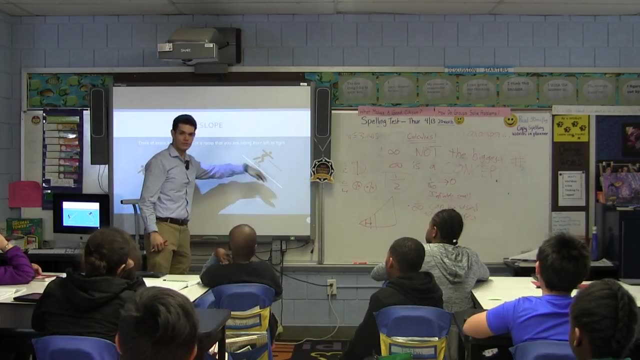 to right. we say that this is a positive slope because he's going up. Now, this guy since, okay, same skateboarder, maybe he got to the top of the hill and he goes: oh, I gotta go down now. Now he's going down this from left to right, So our slope is negative, It's. 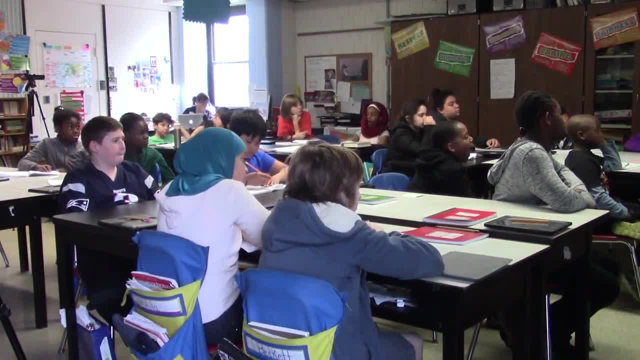 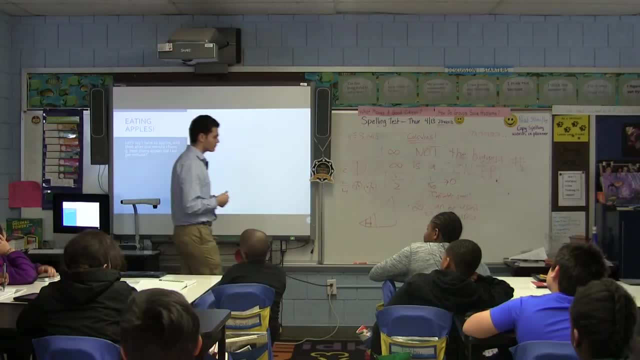 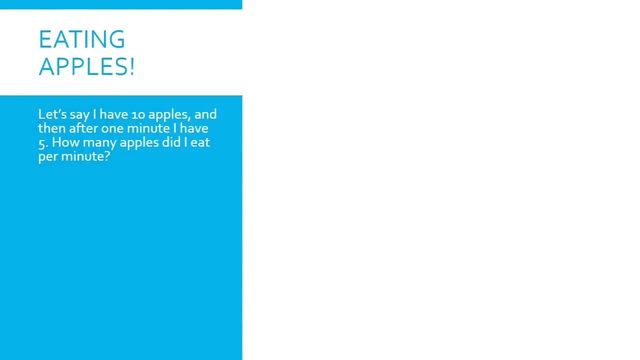 downhill. We understand the difference between those two, Yeah, Okay. So with this, let's move on to talking about apples. Let's say I have 10 apples and I eat. I eat 5 of them in 1 minute because I'm like a speed apple eater. And now I have 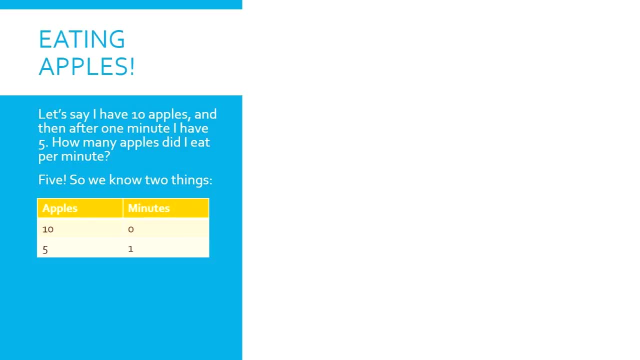 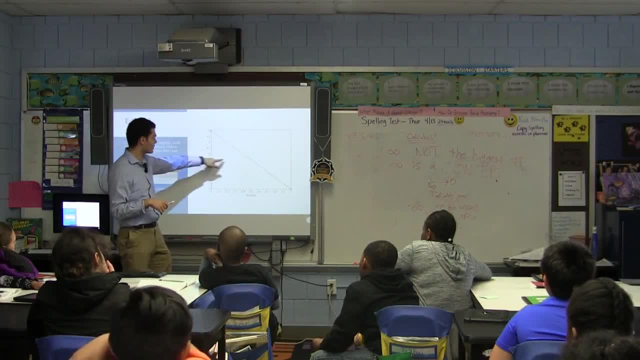 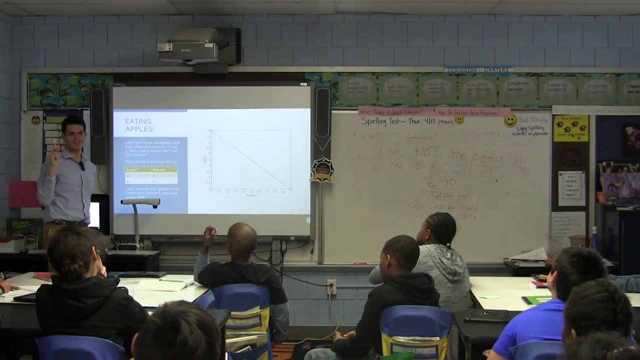 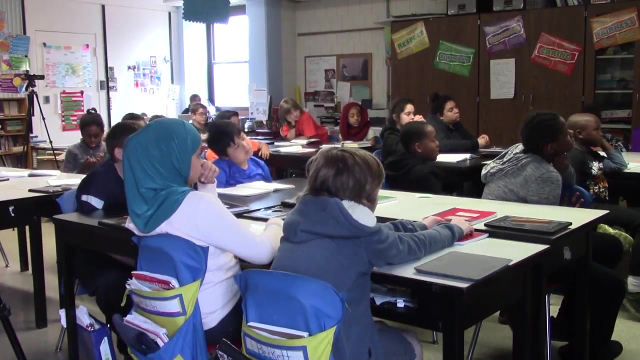 any point on this. on this graph we can read how many apples we have at this minute. So we have this, this line, and what does this look like? Looks like a slope, right, And we can put our skateboarder on it. So this guy is going downhill. so is it positive, or 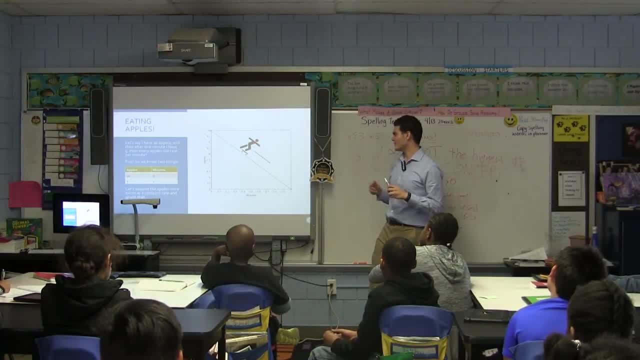 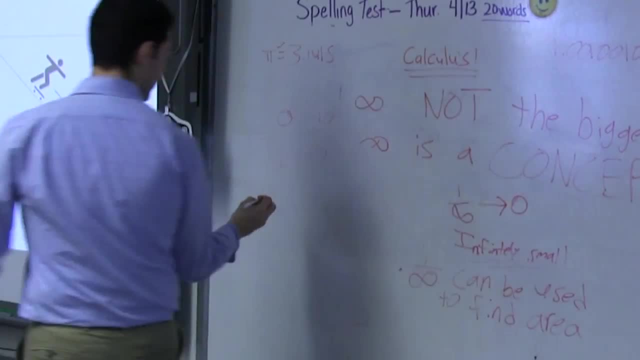 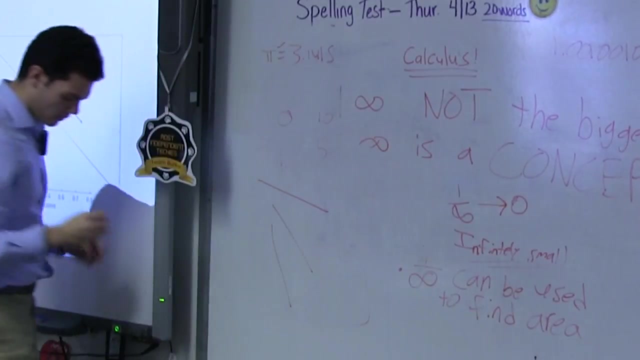 negative, Negative, Negative. But what is the value of this slope We? how can we calculate it Negative And, more importantly, what makes this slope right here? so this line different from this slope or this slope? What exactly is the numerical difference? What's the difference in the actual 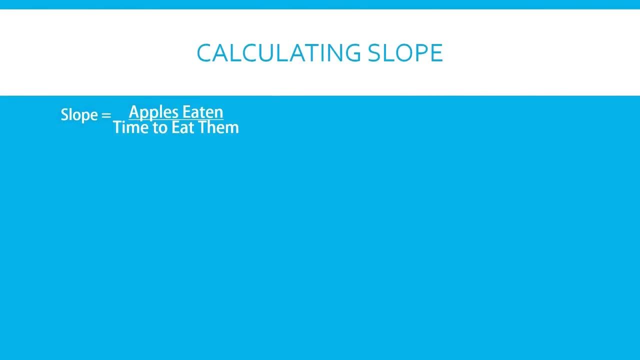 slope between these two, between these three. What we can do is say that the slope is equal to the number of apples that I ate over the time that I ate them. If we have this line, we start at 10, go to 5, how many apples did we eat? 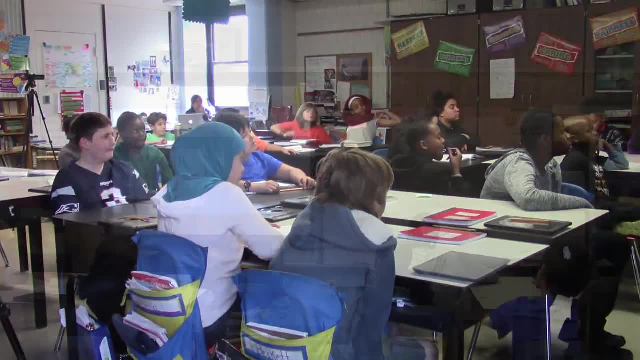 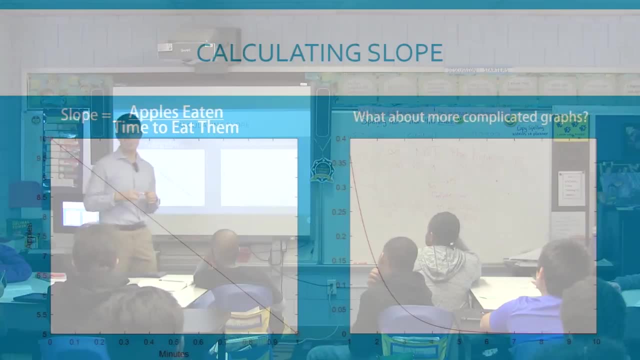 5., 5. And how long did it take? 1 minute, 1 minute. So our slope is going to be negative 5.. But what if we had a line that looks a little more complicated? This isn't a straight line. We have a line that looks something. 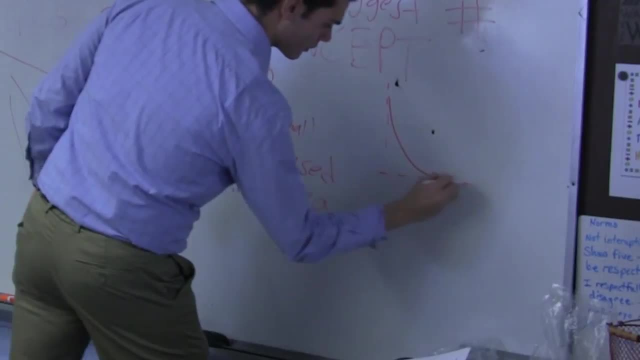 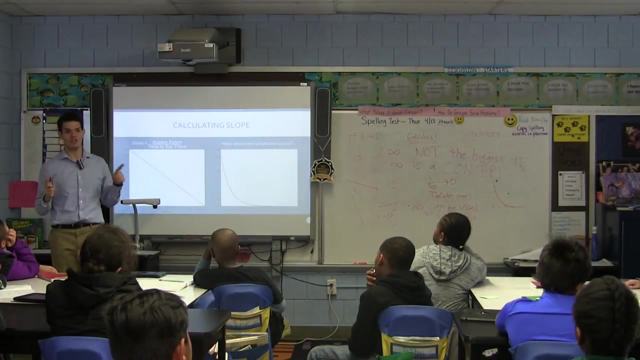 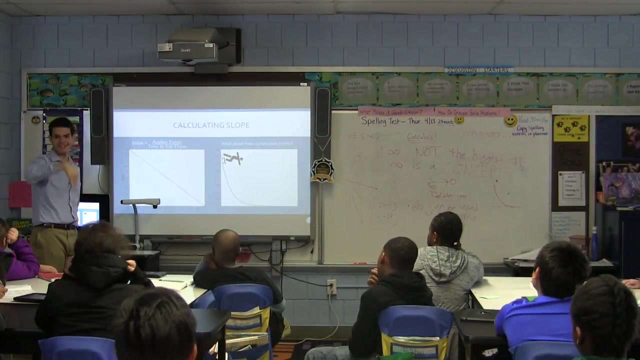 like like this: It's not straight, It's not. it's not easy to calculate that slope And the reason is is because the slope changes. Let's look at a skateboarder here. He's probably going to go really fast Like that's a pretty drastic change. 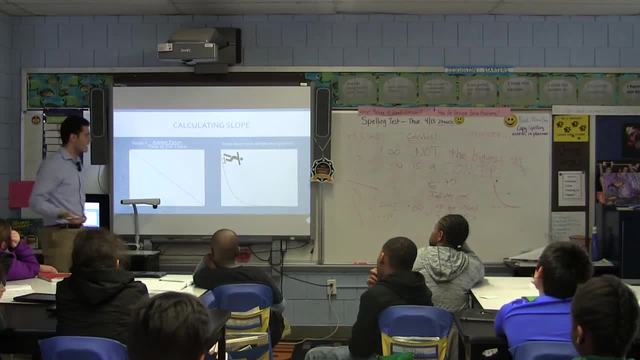 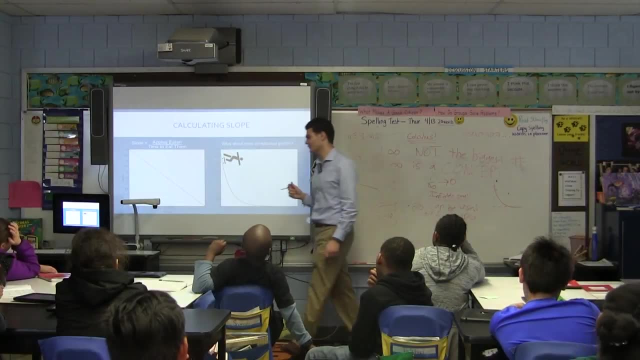 Drop right. It's a really negative slope, Do you agree? Yes, And that let's say that, that that point, that slope is right here. Okay, Pretty negative. And if we put the same skateboarder over here, he's like riding a flat ground. He's not really. 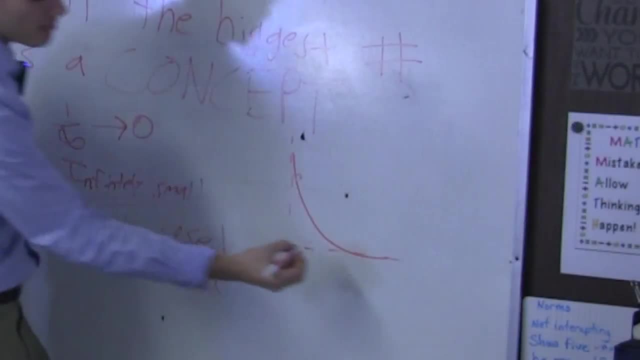 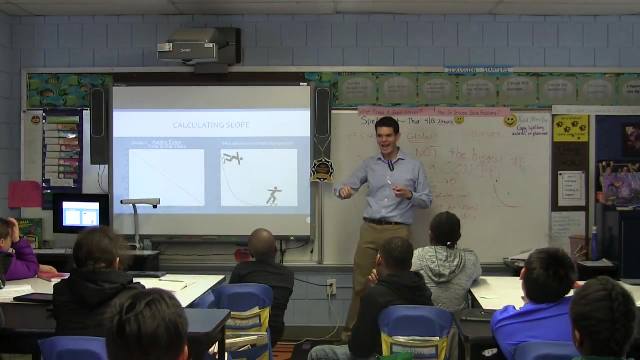 going anywhere, right, He's just, he's coasting, So that slope is maybe somewhere over here, But what's important is that this same graph, this same line, has many different slopes, Because this is different than this, which is different than this, and every single point. 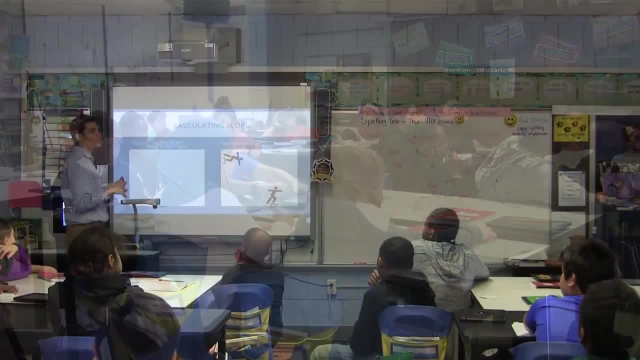 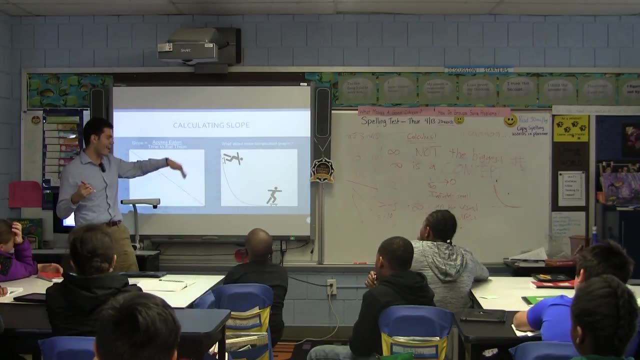 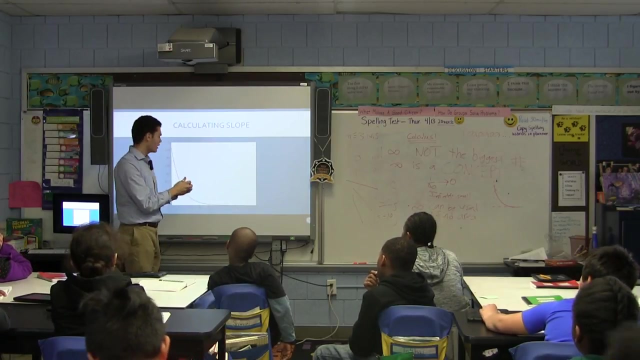 is slightly different slope. So we want to be able to say: well, what is the slope at any given time? Right, How fast is our skateboarder going if we followed this line at any given number? So if we look at this graph and we sort of have it, okay, we take it and we cut it in half. So if you 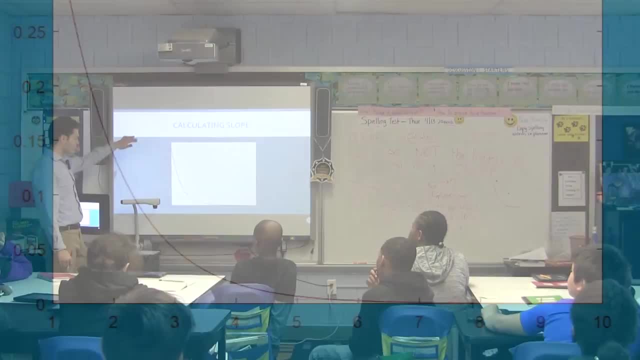 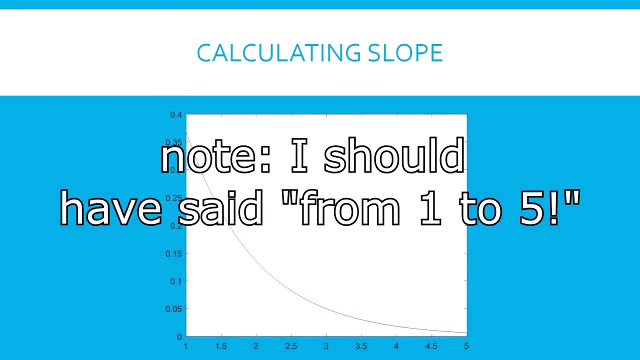 look on the bottom here goes from 1 to 10. And it looks like a pretty curvy line. Now let's say that that's 1 over 1. And let's take a half of that. So now we go from 0 to. 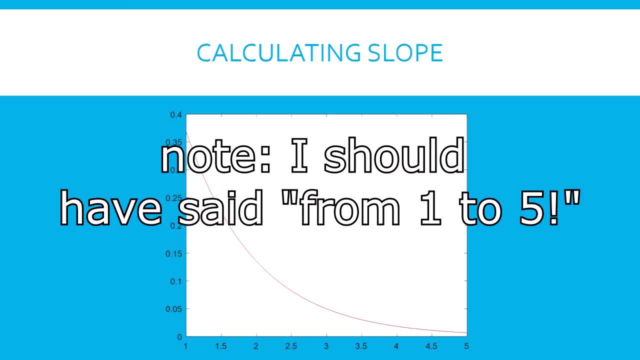 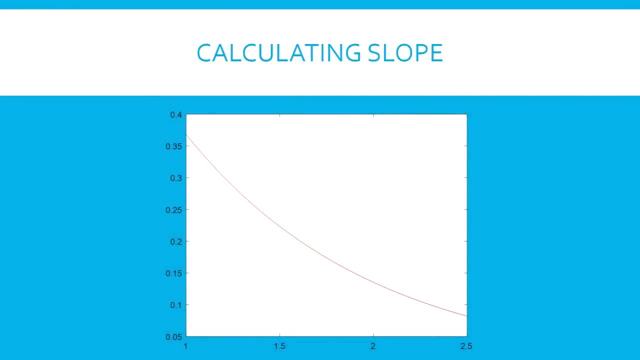 5.. We'll get the numbers on the bottom go from 0 to 5 in our time. Okay, So if we go again now, we go from 1 to 2.5.. Now it looks like an even more straight line. And if we 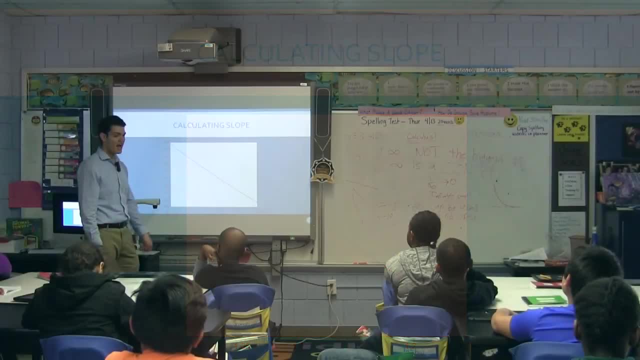 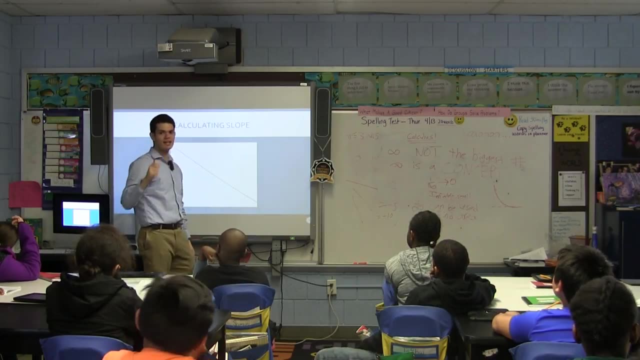 go again 1 to 1.25, that almost looks like an exactly straight line. It's slightly different, It's slightly not straight, It has a slight curve to it, But it's definitely a lot better. And remember, all we did is we went from. 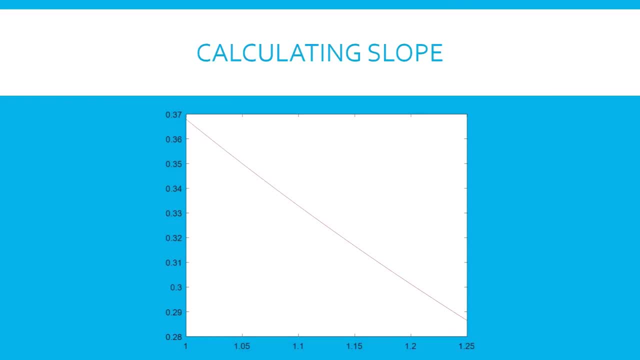 10 to 5 to 2.5 to 1.25.. We kept having that number Okay, And it looked more and more straight. So the question is: what are we doing here? What I would say is that we started. 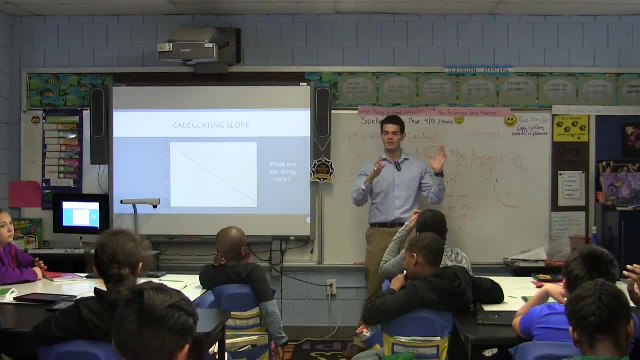 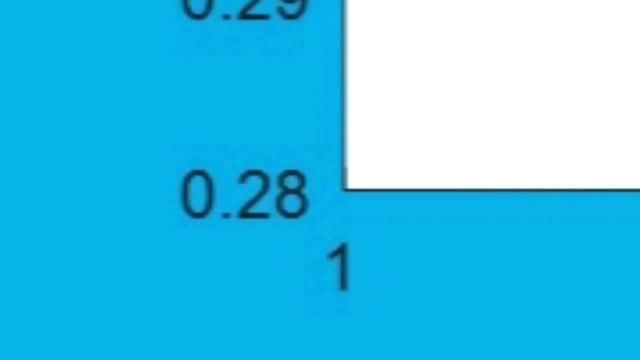 at 1 over 1.. Let's say, we start at 1 over 1, and we have it, We get the 1 over 2.. So now we're at half of our initial graph, centered about 1, because 1 is always there, right? 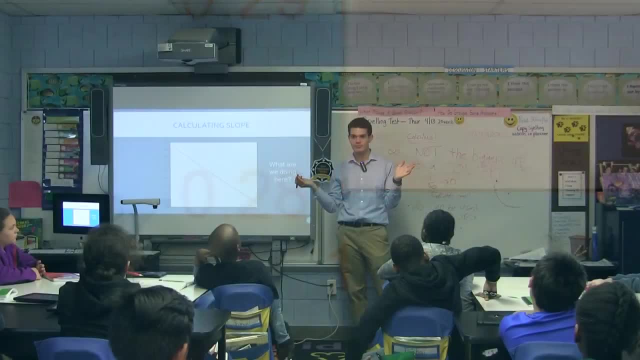 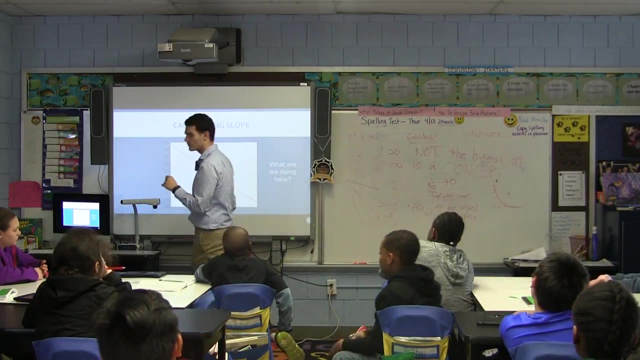 And we halved that. Now we're at 1 over 4.. Are you following me? We're at half of our initial graph, centered about 1. And we're getting. this number on the right is getting closer and closer and closer to 1. Right, So what would happen if? 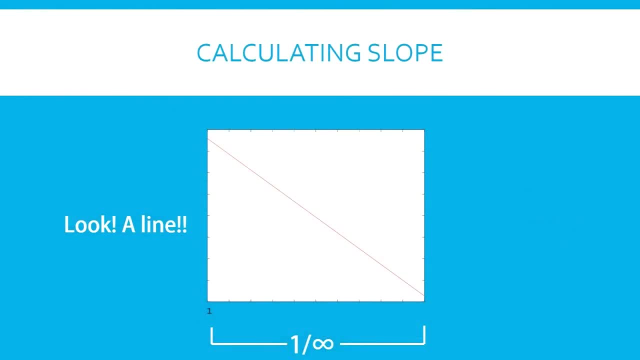 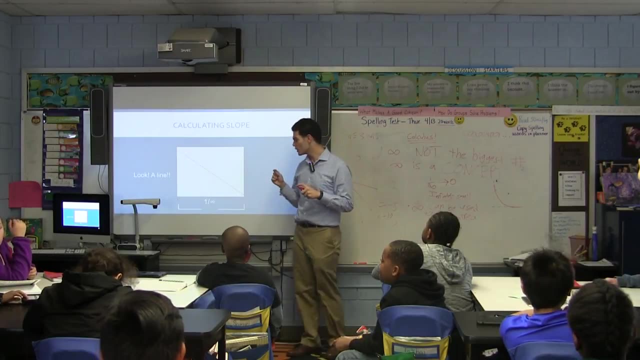 we go a distance of 1 over infinity, It would be a straight line. Remember, infinity is not a number, Infinity is a concept And 1 over infinity is infinitely small. So we go from 1 to 1 plus 1 over infinity, And what we see is we recover a straight line. 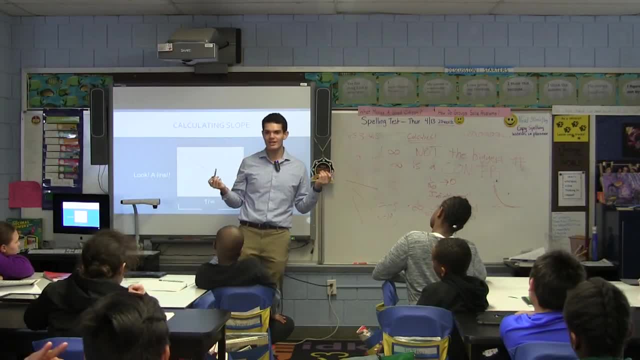 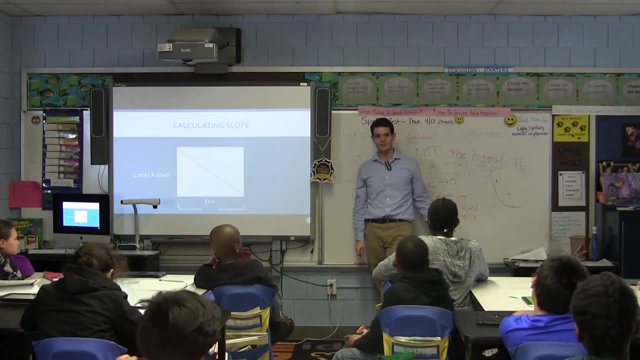 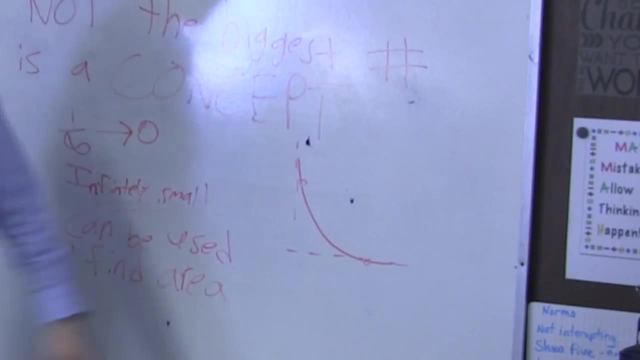 Doesn't that blow your mind? Remember? we started out at this And we said: you can't measure that slope because it's different everywhere. It's different. every single point on this graph has a different slope. But if we have it more and more and we focus in, 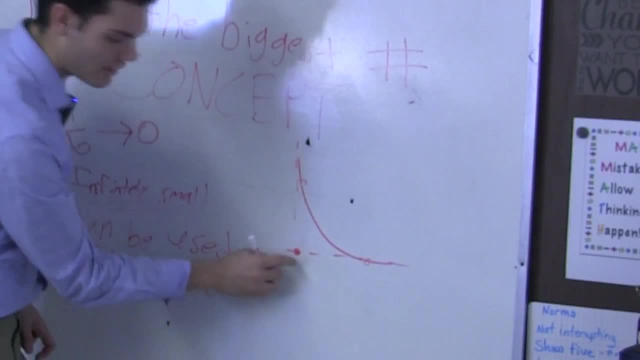 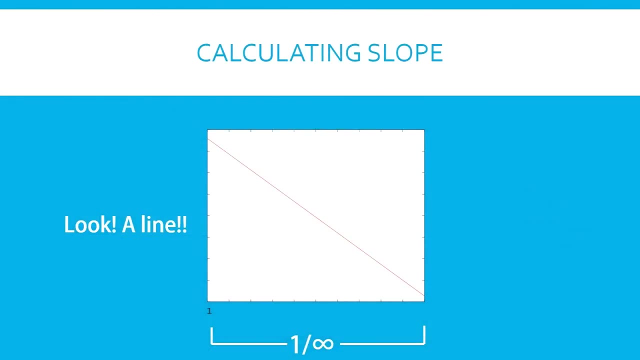 on 1, we focus in right here, We're focusing on this time And we look at only that instant of time. it looks like a line. We said before that every single point has a slope And we also said that in order to. 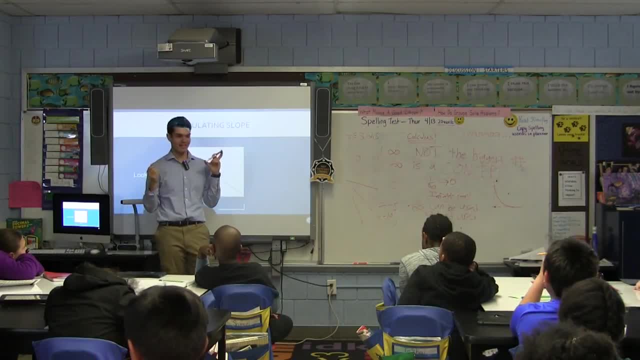 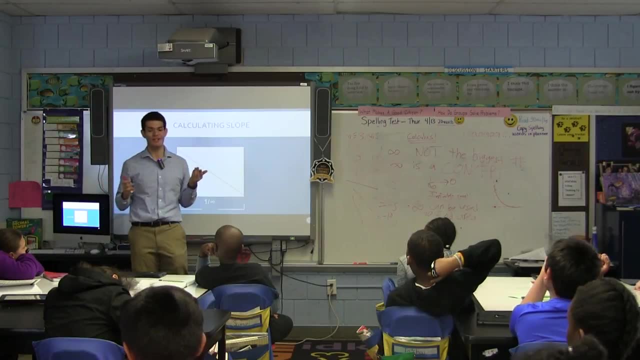 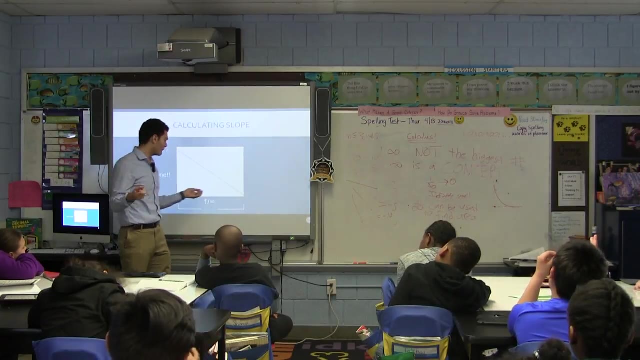 measure that slope, we need a straight line. So if we look at an instant in time- that is essentially just one point- we'd better get a line, because we need a line to measure the slope there, Do you agree? Yeah, So this makes complete sense If we look at a time from 1 to something just after 1, infinitely. 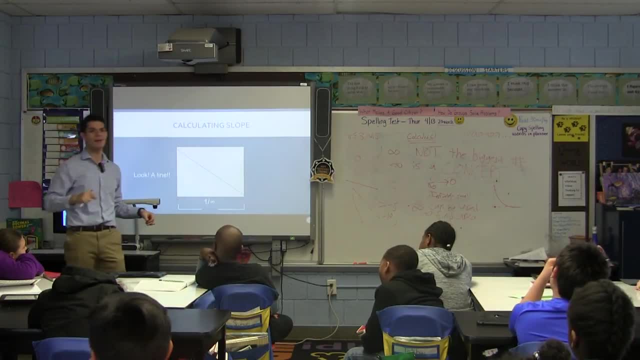 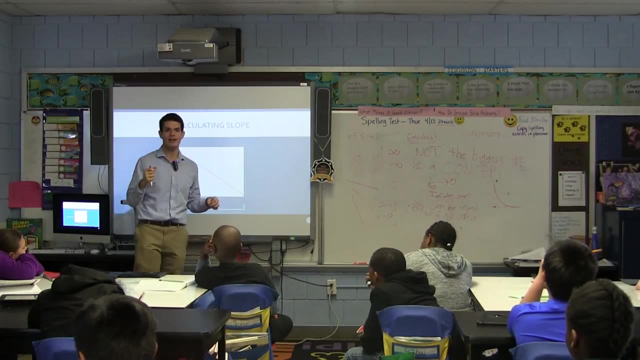 close to 1, it better look like a line, because we want to be able to measure that slope, because we know it exists, And that's important is that we know the slope has to exist. So there must be a line there. And the question is: 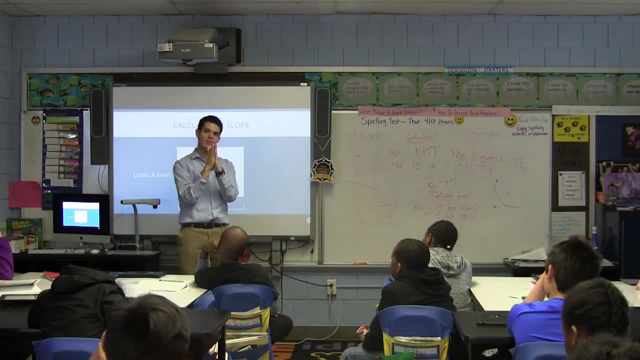 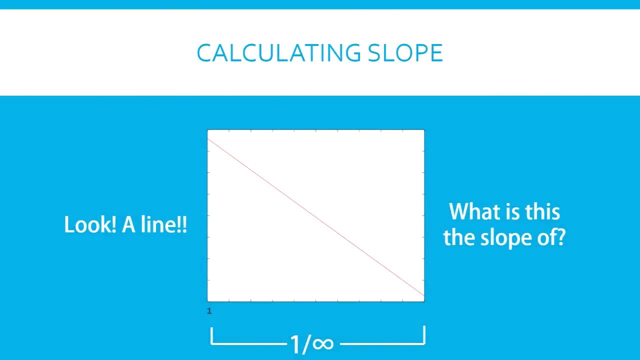 how we have to just be able to look only at that point in time to find that line. And this is very important because we can measure the slope of this line Based on this picture. we know that it exists and we know that it's calculable. We know 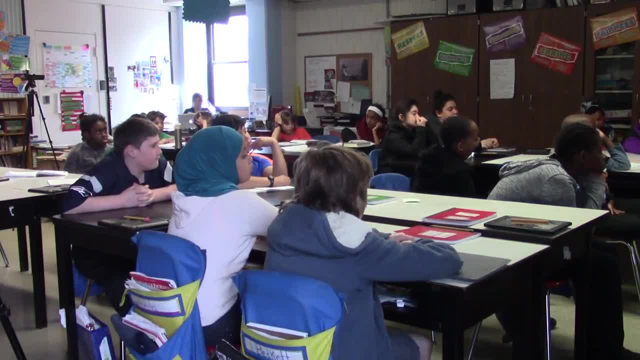 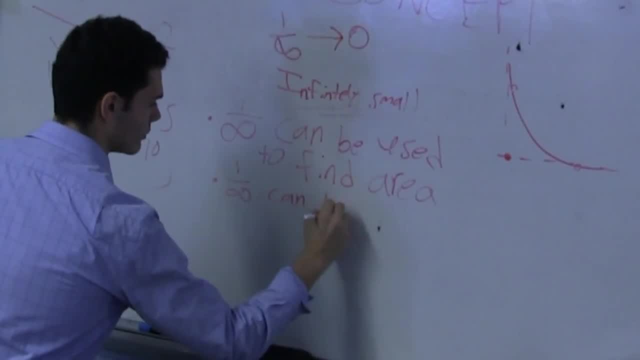 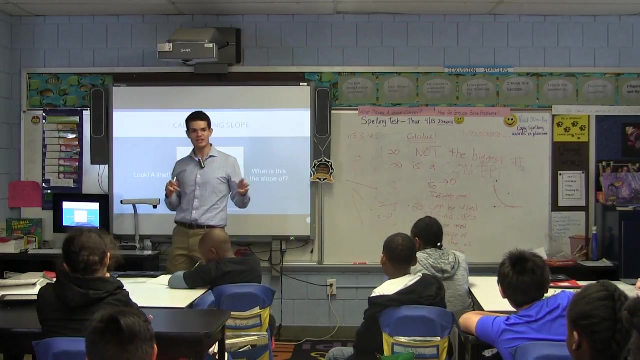 that we can find it if we have the right tools. I want you to leave with this idea That 1 over infinity can be used to find the slope of a curved line, And this is also crucial. Remember how I said the area was one of the two central ideas of calculus. 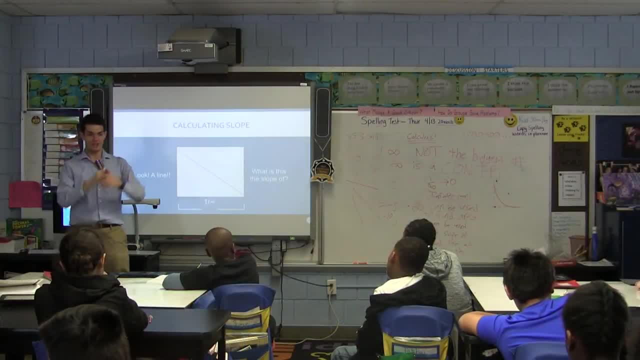 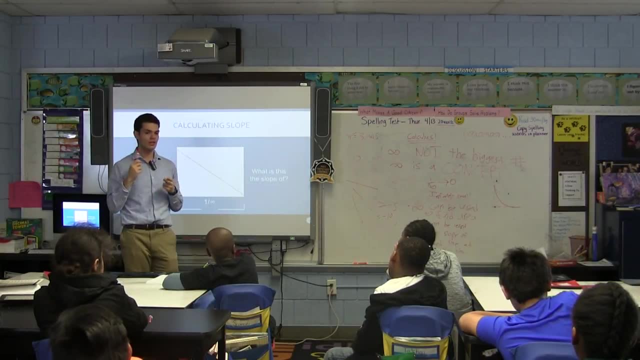 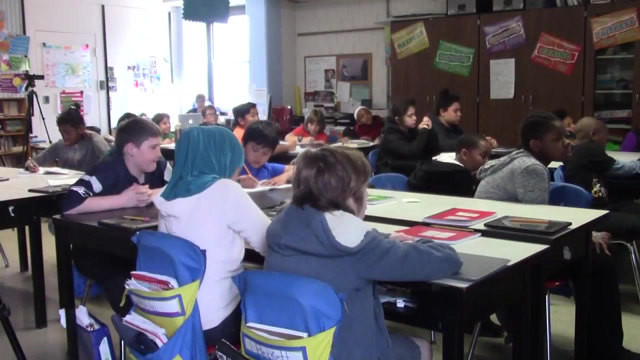 This is the other one. This is the second half of the complete picture of calculus. We can use calculus to not just find the area of a shape, but to find the slope of a function of a line, of a graph that otherwise we wouldn't be able to find the slope of. 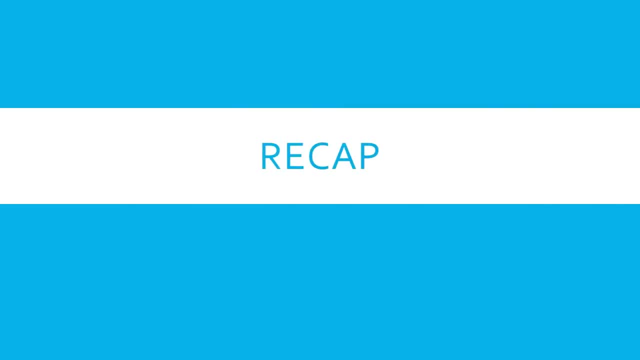 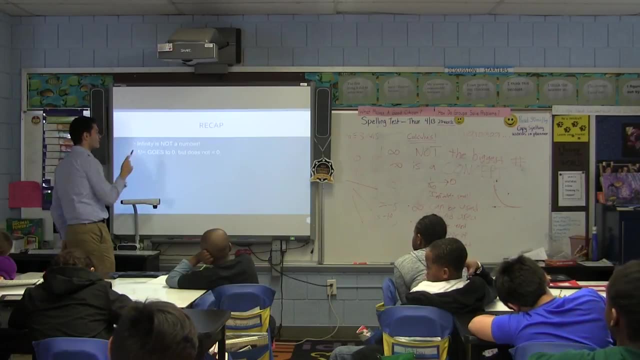 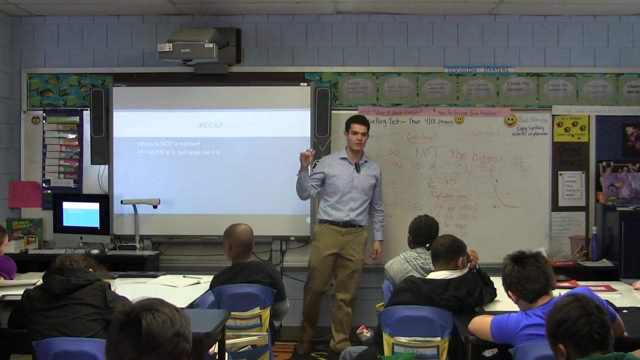 All right. So let's just recap what we learned today. We learned, most importantly, that infinity is not a number, Infinity is a concept. And we also learned that 1 over infinity is not equal to 0.. It leads to 0.. It goes to 0.. If we look, 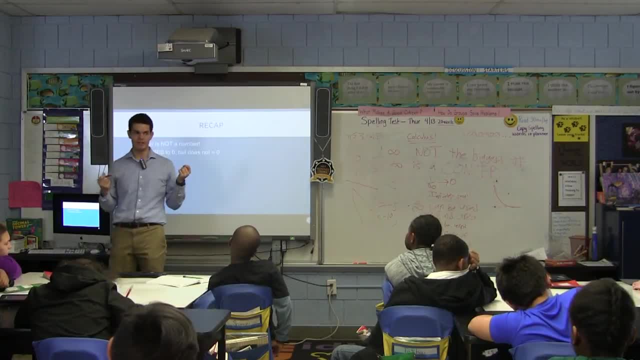 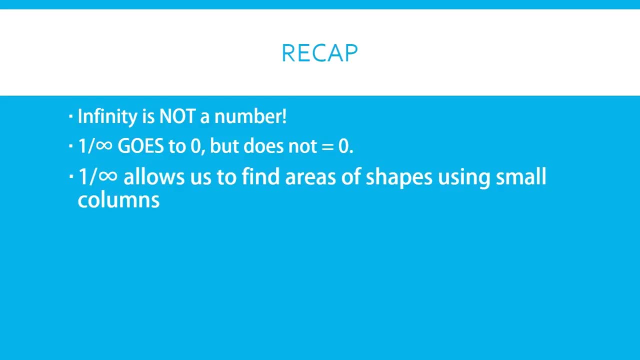 1 over infinity. it gets smaller and smaller and smaller, becomes infinitely small and goes to 0.. And 1 over infinity allows us to find the area of shapes using really small, infinitely small columns, which is crazy. If I give you a weird object, like maybe I give you 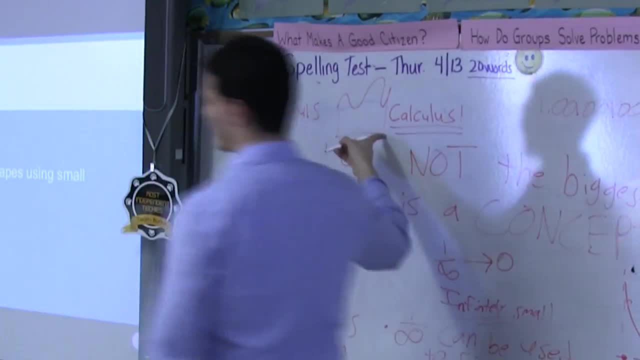 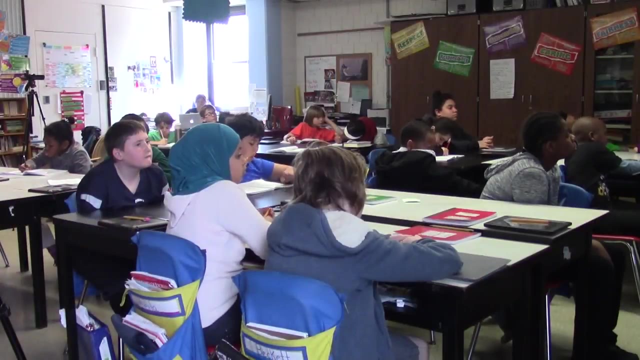 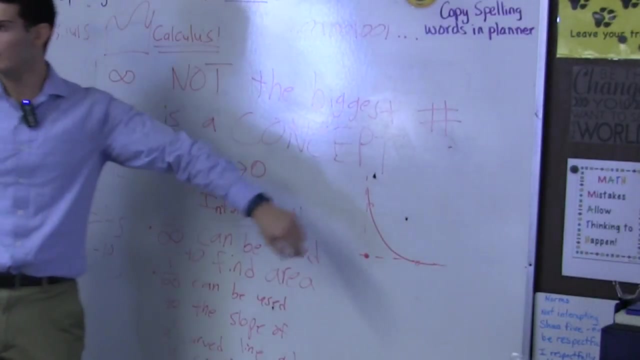 something that looks like this: how do you find the area of that thing? That's pretty hard, right. You want to have a formula for that. We want to be able to use the columns. We also showed that 1 over infinity allows us to turn a curvy line. a curvy line like this: 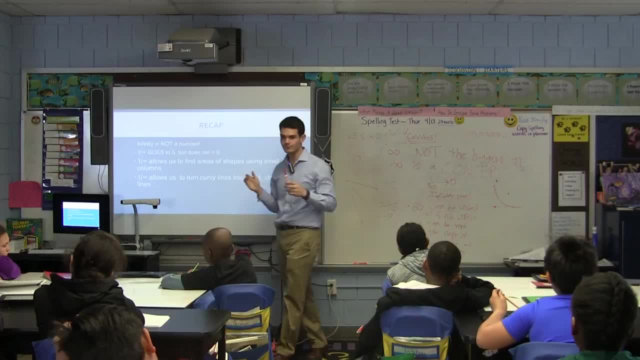 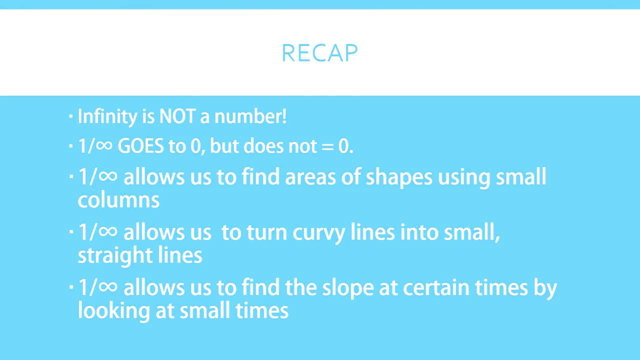 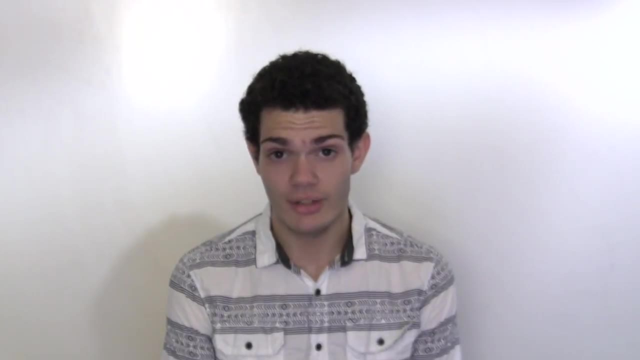 into a straight line at a specific point at a specific time, which is amazing because it allows us to find the slope, at any given time, of a line that we normally wouldn't be able to. Students just beginning to study calculus always find the concepts of limits, derivatives. 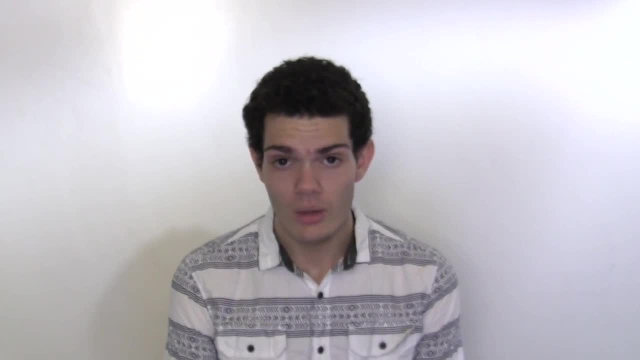 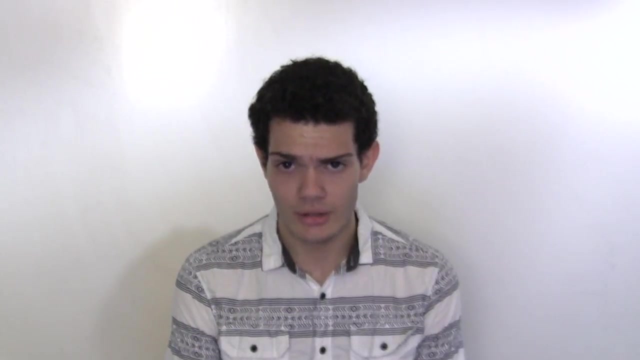 and integrals hard to understand, But when these concepts are broken down and explained in new, unique ways, such as by using coins to visualize integrals, they become infinitely easier to understand. In fact, the rather unconventional methods for teaching calculus used in this video 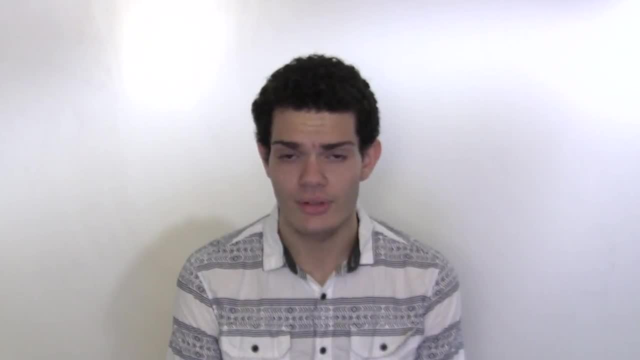 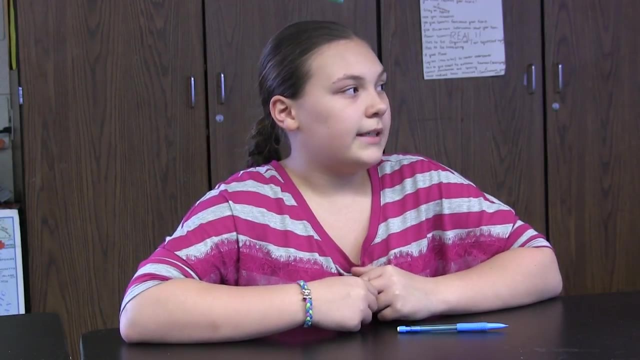 allow the same students who usually hate things like word problems to follow these daunting concepts. You were actually really really good at explaining everything. You gave a lot of details and I think that was really good. It made sense Like I could understand it. 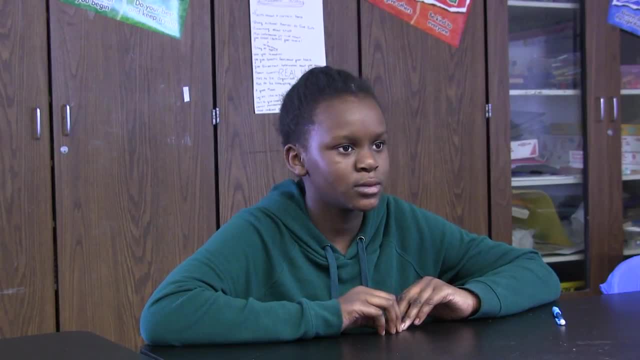 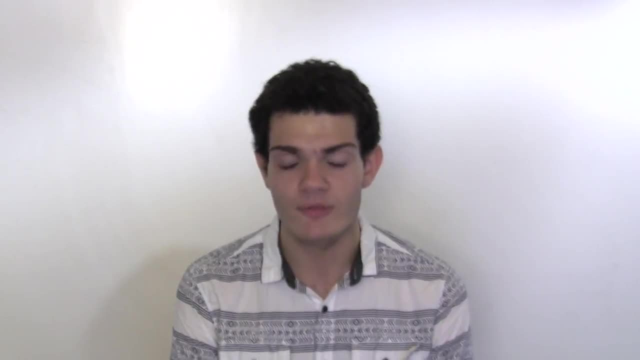 It made it easy to understand what you were trying to say. So next time you hit a roadblock and want to give up because you just can't grasp a concept right away, take a step back and try to tackle the concept in a new way. 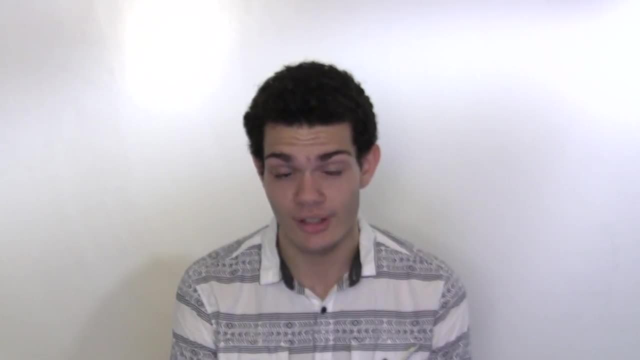 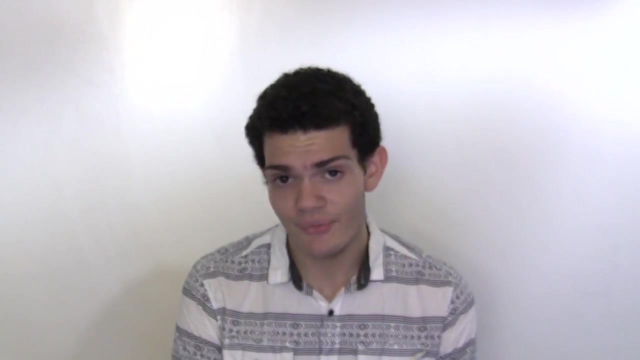 just like we did with using pizza to explain infinity and skateboarders to explain slope. Then, once you dive into the awesome fields of mathematics, you will just like the fifth figures in this video. Summer, I want to ride a bike. I want to learn about like molecule structure. 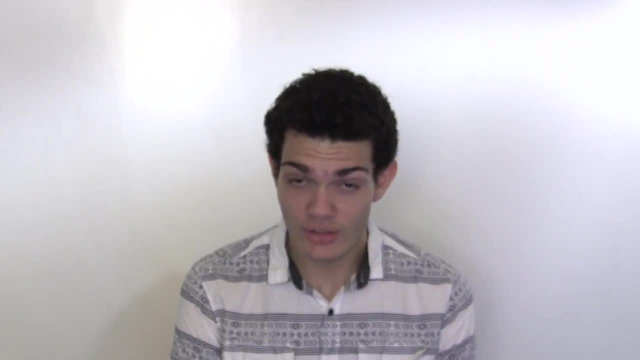 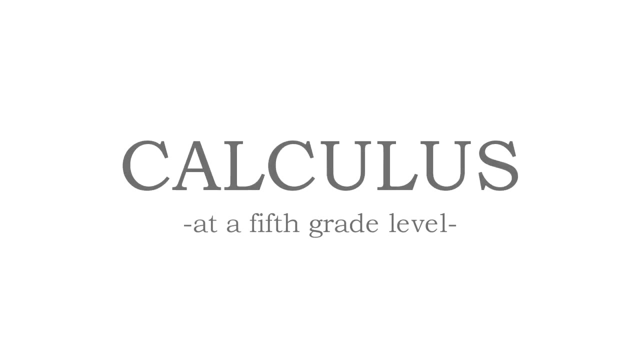 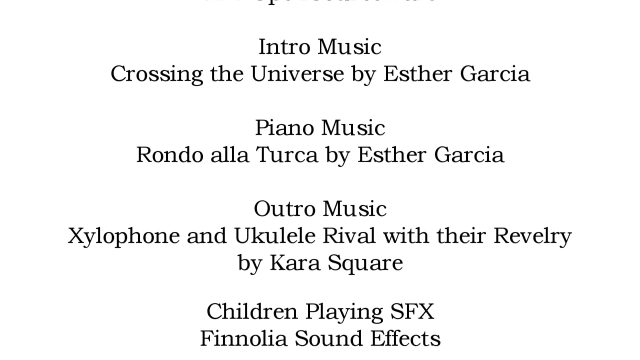 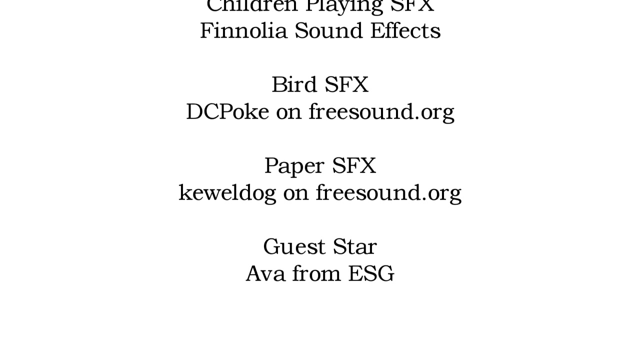 Have a thirst for knowledge and one day, just like those students, go on to change the world. See you next time.